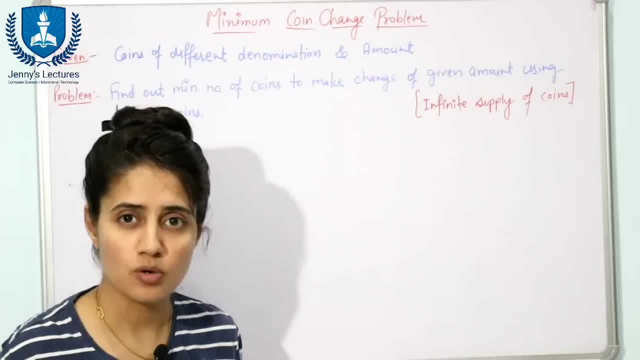 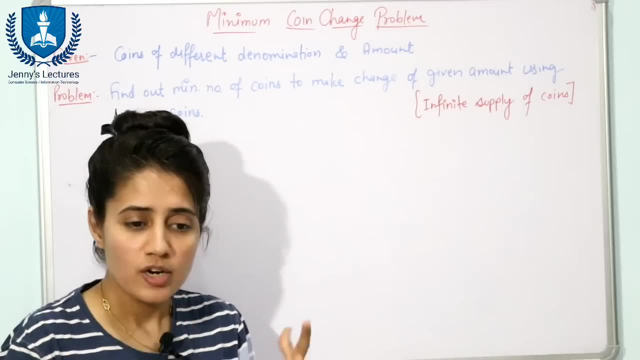 the help of dynamic programming. only. See, this is kind of optimization problem. What are optimization problem? I have discussed when we were discussing the basics of dynamic programming. See, those kind of problems in which you are going to find out either minimum or maximum solution of the problem. 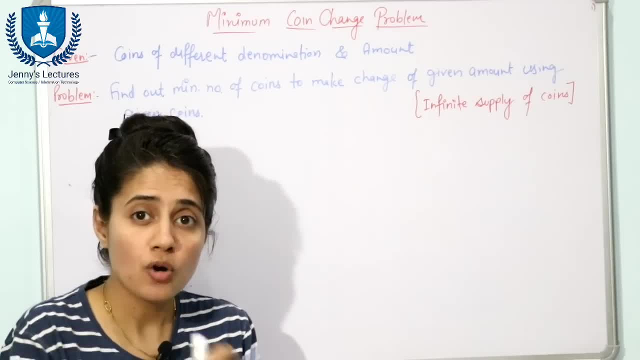 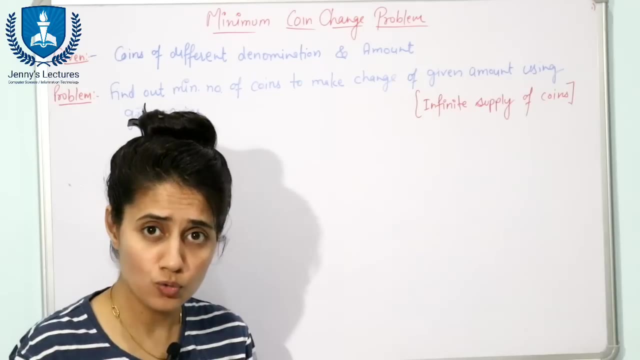 Means. see when you find out that minimum, maximum, shortest, longest total number of ways, these kind of keywords in the problem, then you can see that those kind of problems are optimization problem. So both greedy method and dynamic method can be solved, can be used to solve. 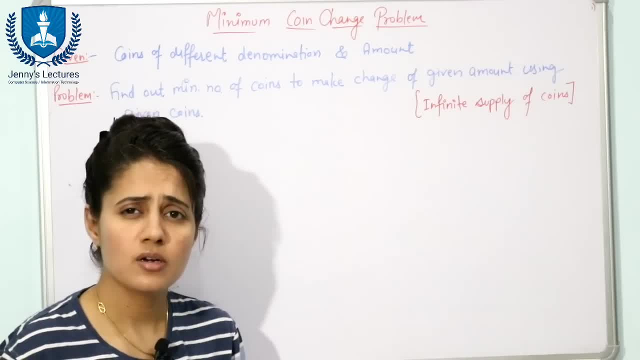 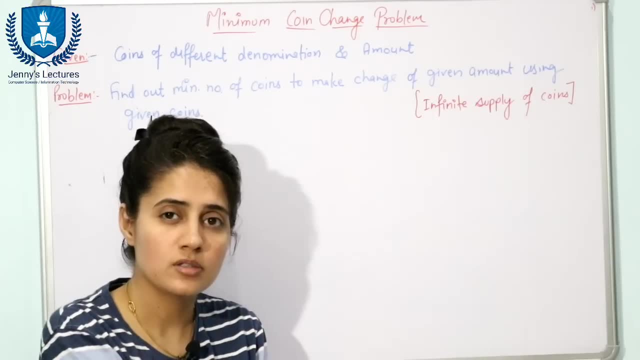 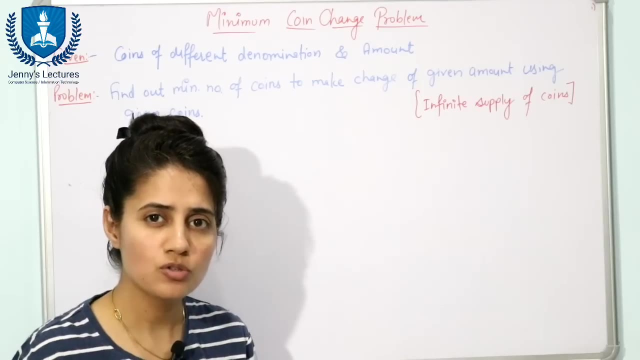 optimization problem. Fine, And obviously we can solve those problems with recursion also. I have discussed the drawbacks of recursion and why we use dynamic programming over recursion In that video only when we were discussing the basics of dynamic programming. I will provide you the link in the description box. You can check it out there. Okay, Now see. first of all I will discuss: 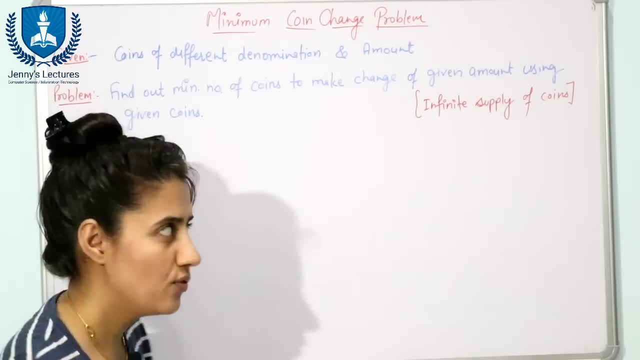 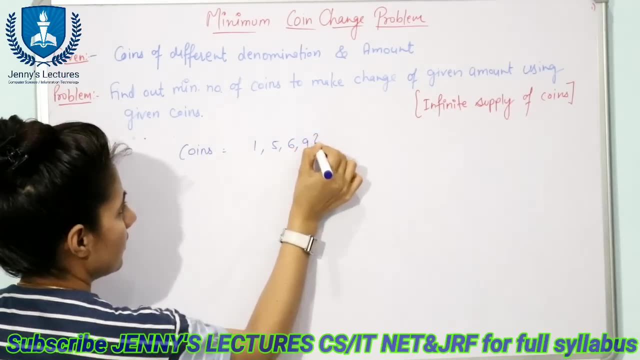 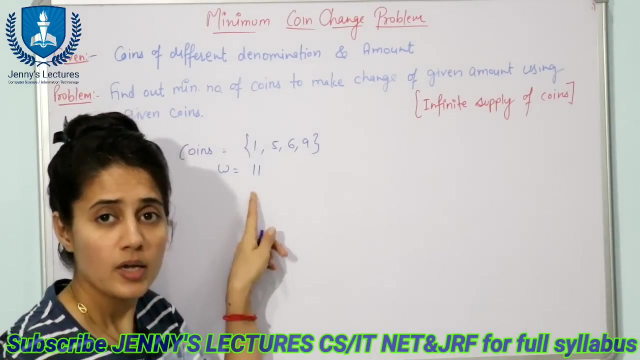 what are the drawbacks of greedy algorithm? Fine, Let us take one example. Suppose we are given these coins- 1,, 5,, 6 and 9- and sum, or you can say this amount is given as 11.. Okay, Now you have to. 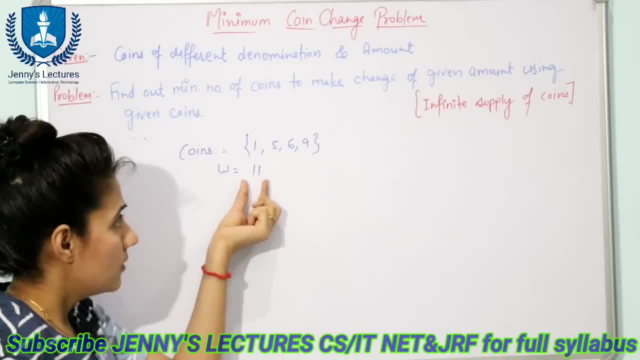 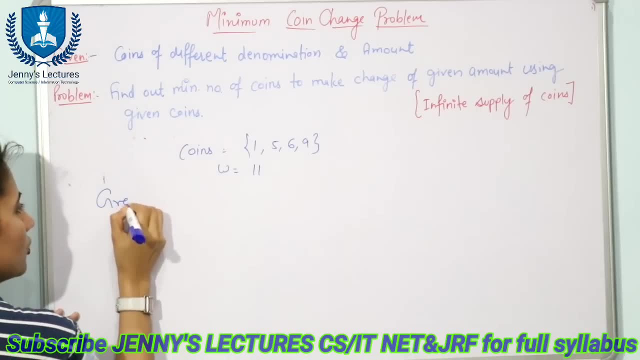 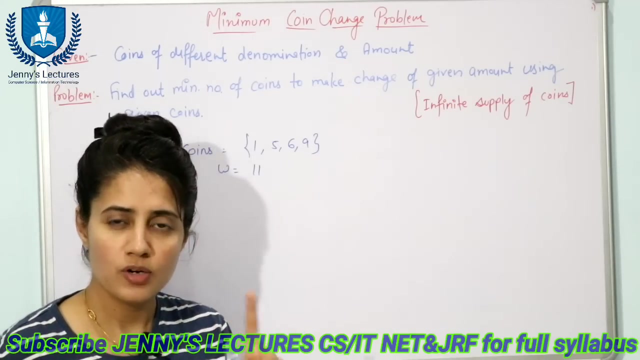 use minimum number of coins to make this change. or you can say: to make this sum with the help of these given coins. Now, if you apply that greedy approach, what are the steps in this greedy method? See, let us take one example. I have one rupee coin, one 5 rupee coin and one 50 rupee coin. 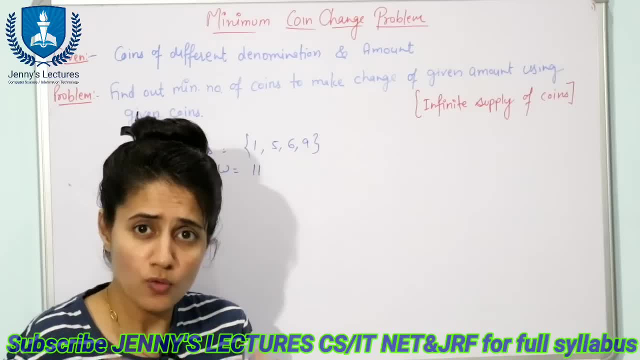 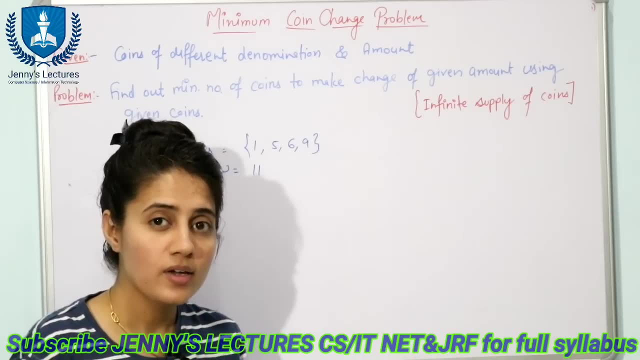 Now, if someone is, I am offering one of those coins to someone, and if that person is greedy and if I give him the choice to choose from those coins, then what coin or coins of which denomination he will choose? Obviously, if he is greedy, then he will choose what 50 rupee coin. 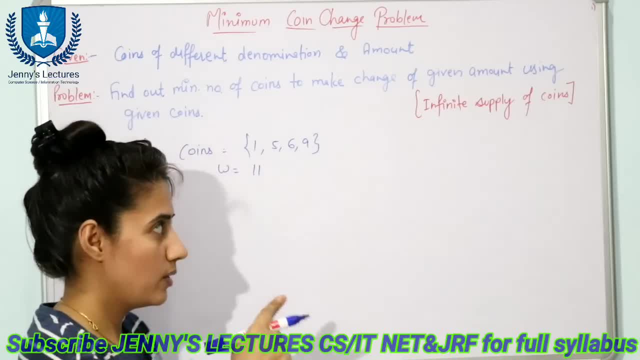 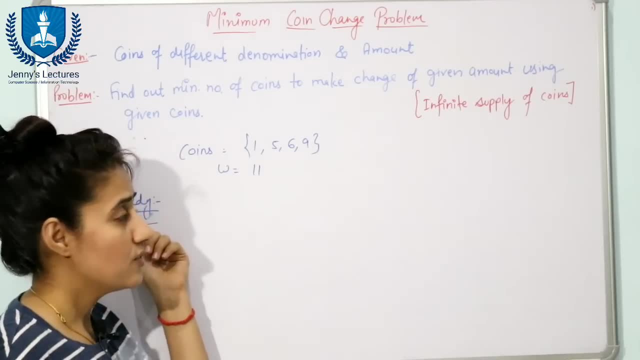 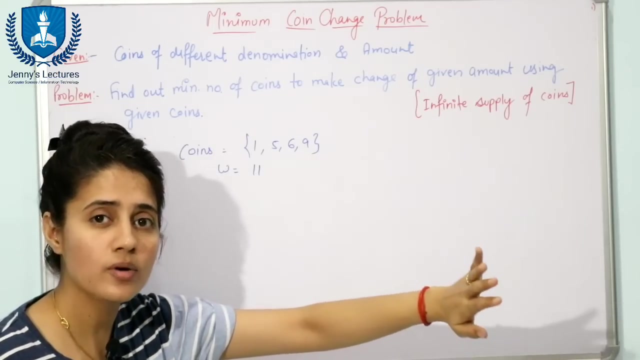 Fine. So that simple formula has to be applied in this case also, Whatever we apply in real life. Okay, See now. in this case, first of all, we will choose the highest denomination, but that highest denomination coin, but that coin should be either less than or equal to this amount. 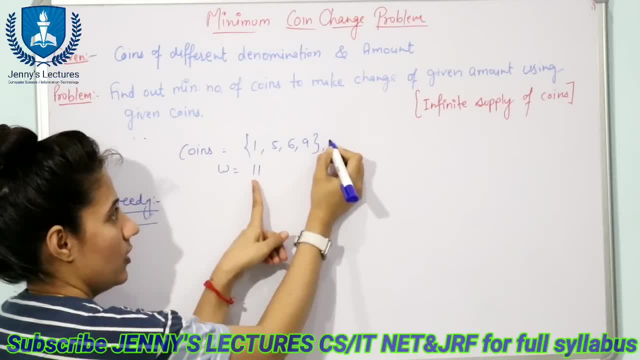 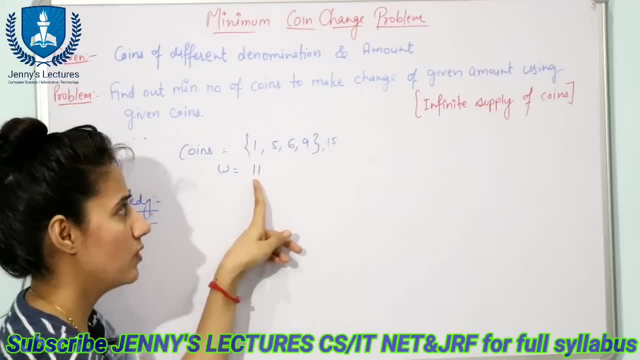 We can't say that if we are having one more coin or that one is having a 50,, 15 denomination, So we cannot choose this one. In greedy also, we cannot choose this 15, because the sum is what 11.. So 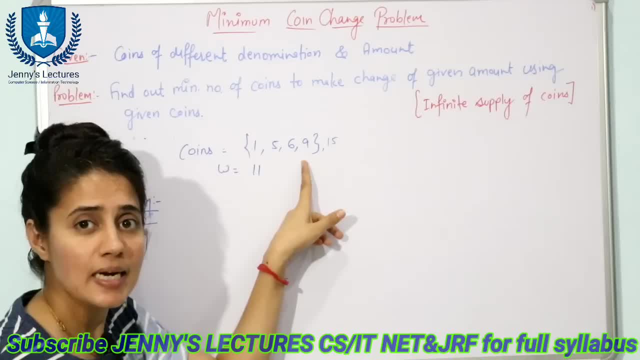 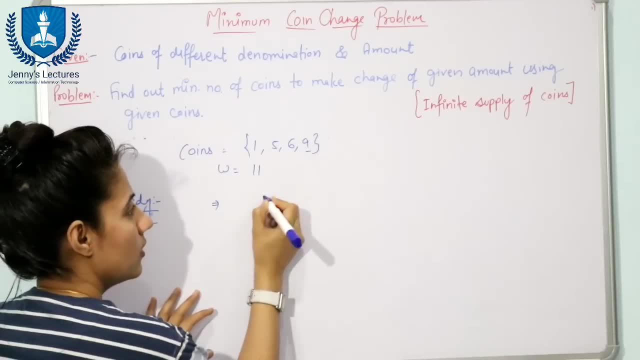 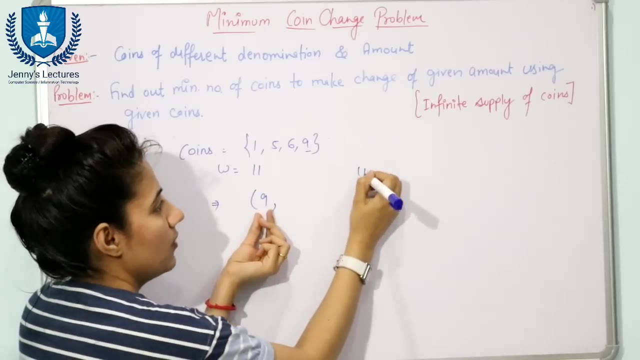 we have to choose the highest denomination coin, which is either less than or equal to this sum. Okay, Now, according to greedy, what we will choose first, We will choose what 9.. choose what 9? okay, now we have taken this 9. the remaining amount is what? 11 minus 9, that is. 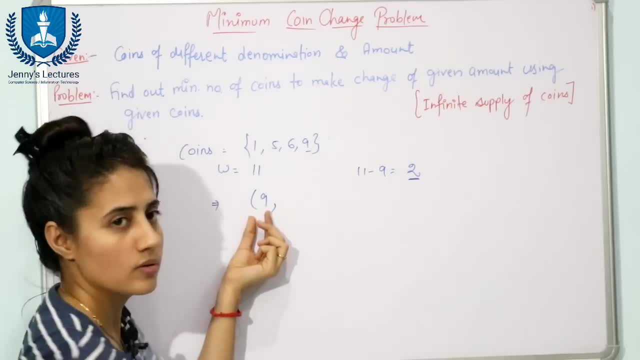 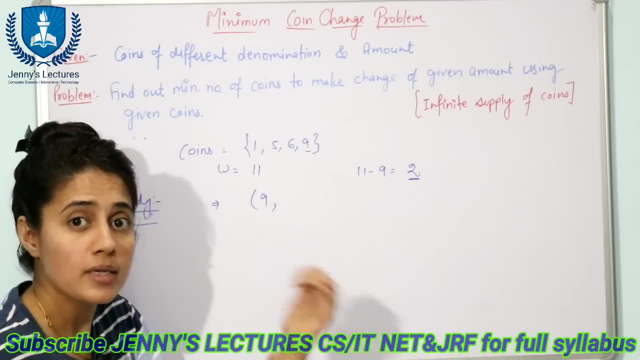 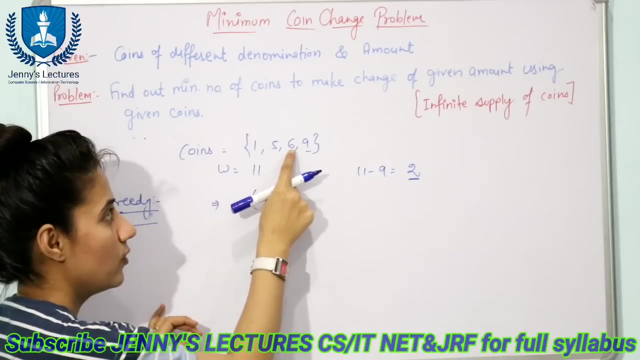 2. now you have to make this amount using these coins. now again, you will apply that first step: choose the highest denomination coin, but that should be either less than or equal to this sum. now, which one you can choose? you can choose only one. you cannot choose 5. you cannot choose 6. you 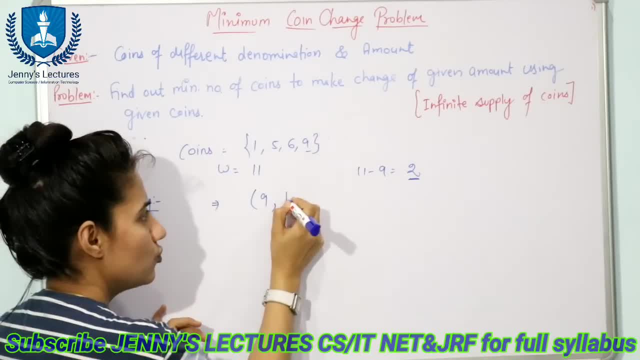 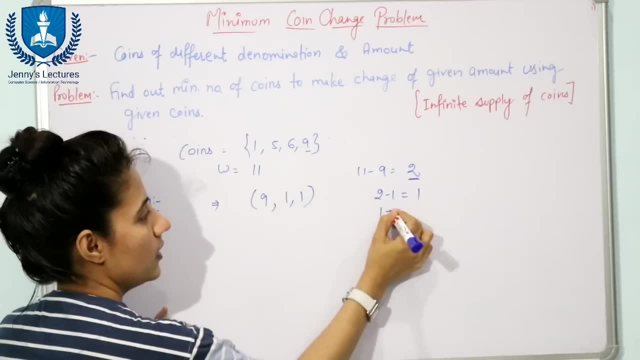 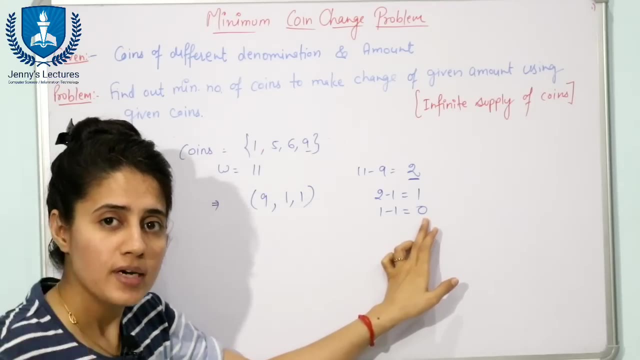 cannot choose 9 because these are greater than the sum. so if you choose one, then remaining sum is 2 minus 1, that is 1, and again we will choose 1 and remaining is 1 minus 1, 0, and this this steps would be followed till we find the sum 0. now, according to greedy approach, how many coins you 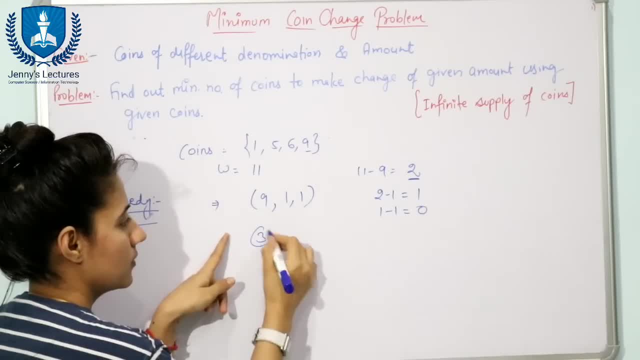 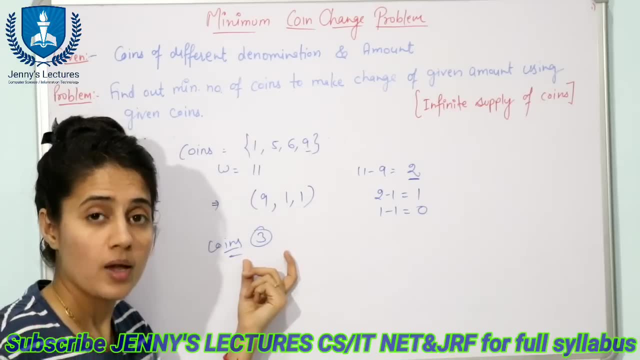 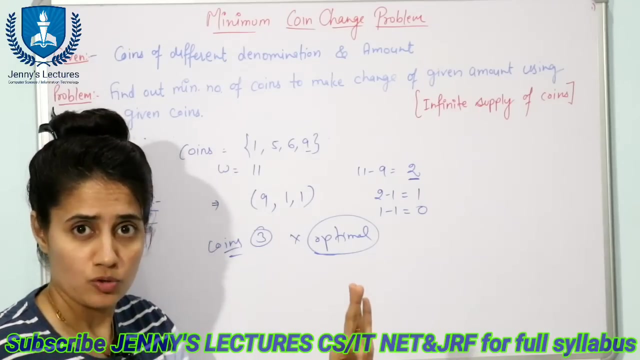 need to make this sum 1, 2, 3, 3 coins right: 2 1 rupee coin and 1, 9 rupee coin, 3 coins. you need you, but this is not optimal. this solution is not optimal solutions. why so? because if, if we choose, 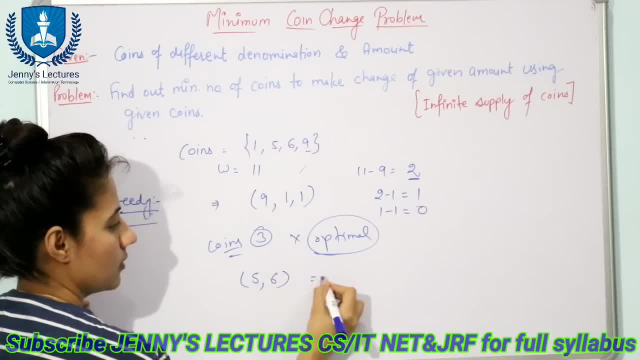 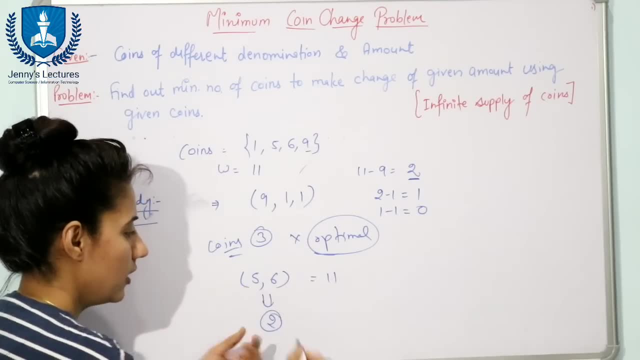 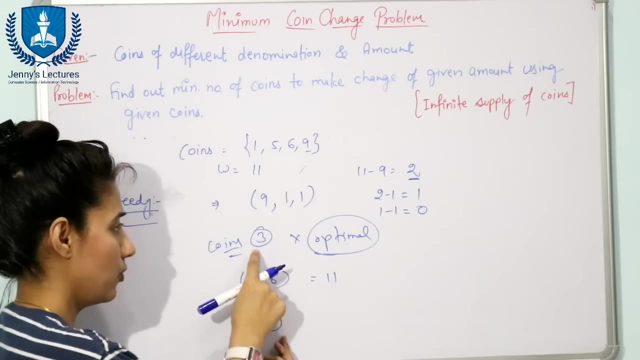 one five rupee coin and one six rupee coin. then also you can make a sum of eleven. and in this case, how many number of coins? you need only two. and according to greedy, how many coins? you need: three. how many. minimum number of number of coins: three. so sometimes greedy approach will not give. 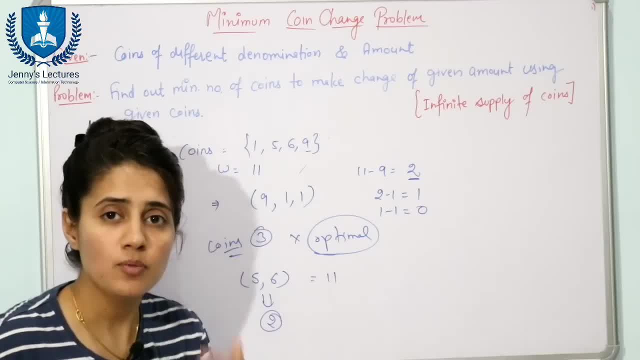 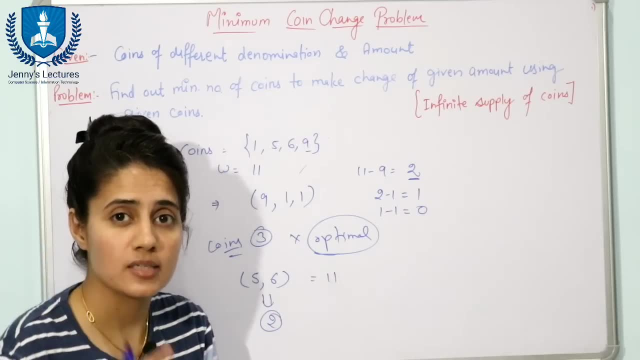 you the optimal solution. but if you apply dynamic programming then it will guarantee give you the optimal solution if the solution exists. the condition is, if solution exists, then dynamic programming will give you the optimal solution. that is for sure. okay, that is why we do not use greedy approach in to solve every kind of optimization. 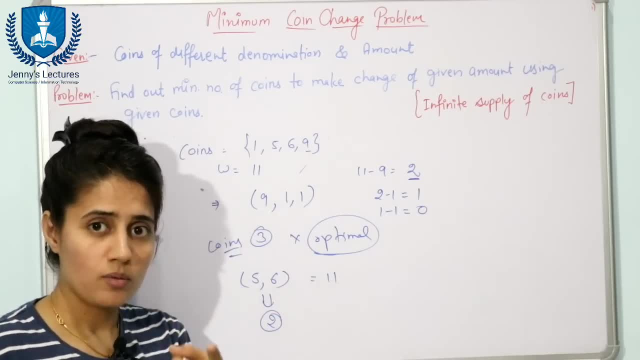 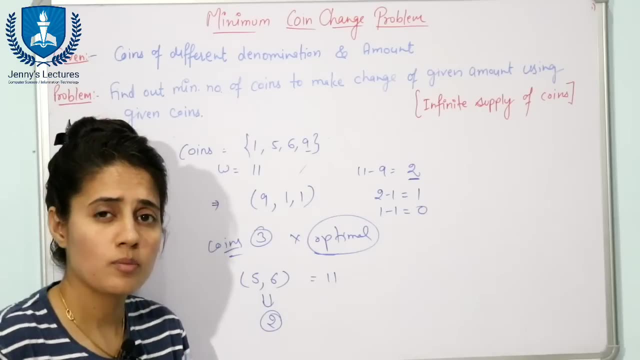 problem. okay, and i guess in korman it is given that which kind of problem can be solved using ready and which kind of problem can be solved using which kind of optimization problem is best to solve with dynamic programming. see, this kind of problem can also be solved using recursion. 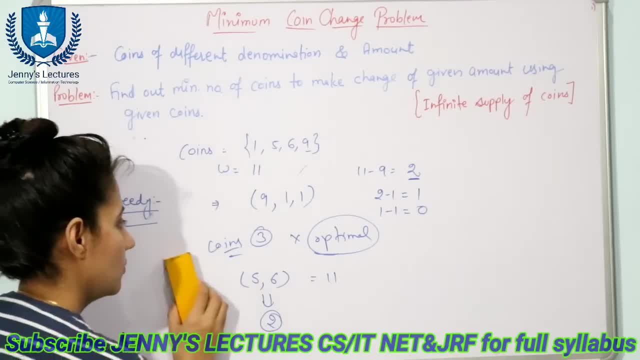 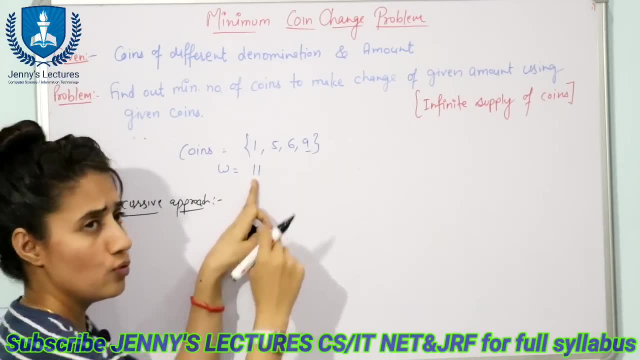 but some drawbacks of recursion are there. i will show you how. now, if you apply that recursion, or you can say recursive approach, then what? what is the thing? suppose i am taking you are, you are going to make the sum of this eleven. so i am taking the sum of this eleven, so i am taking. 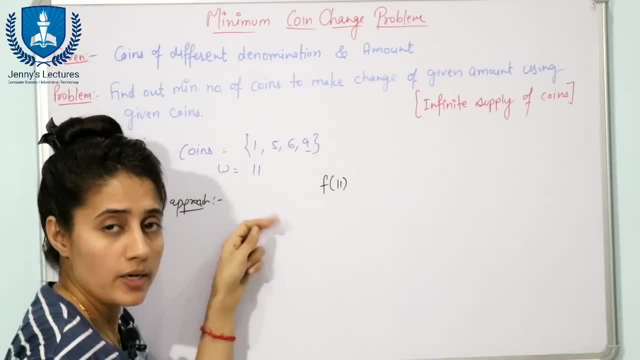 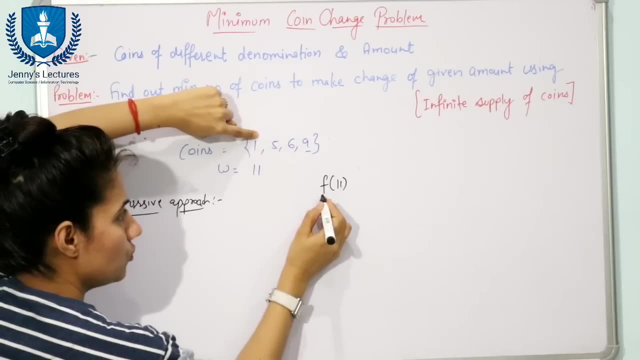 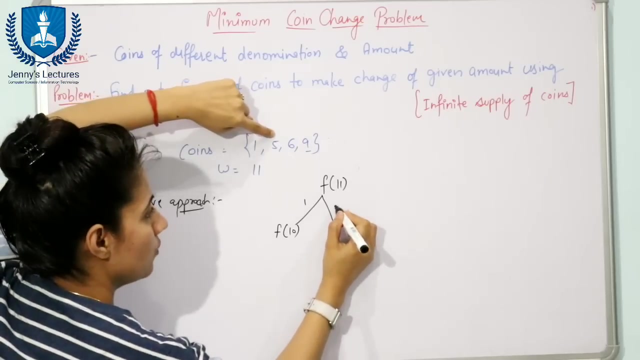 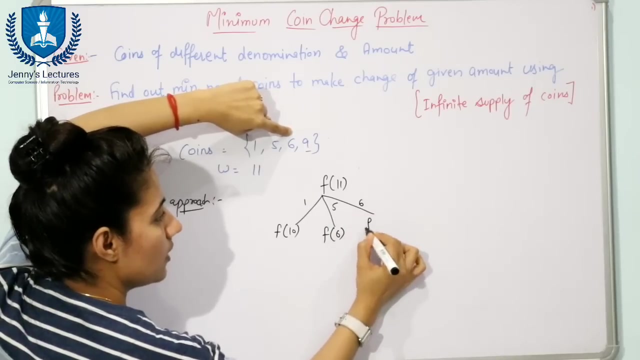 function of 11.. now, in recursion, what what we have? at starting, we have four choices. you can choose one, if you. if you choose one, then remaining amount is 11, 1, 10.. or second choice is: if you choose 5, then remaining amount is 11, 5, 6. if you choose 6, then remaining amount is 5 and if you 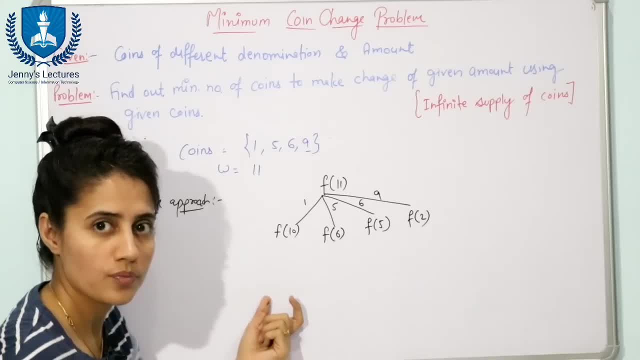 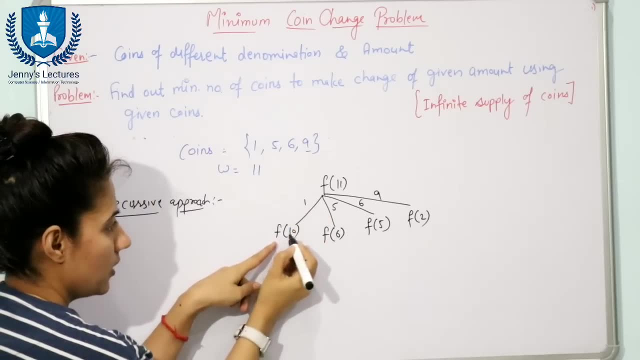 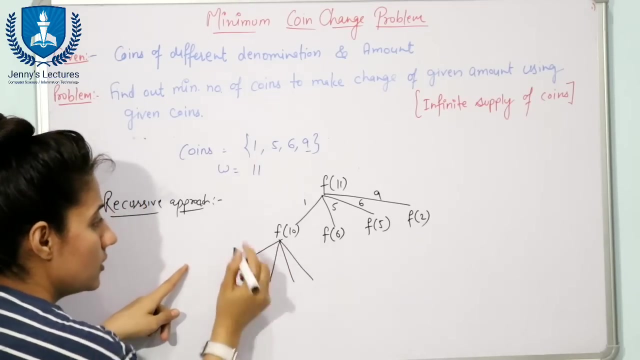 choose this 9, then remaining amount is 2.. so we have four choices here. now again in the next step, suppose, if we are, if we are going to this path, then we have reached here. here also we have four choices. here also you can choose either: 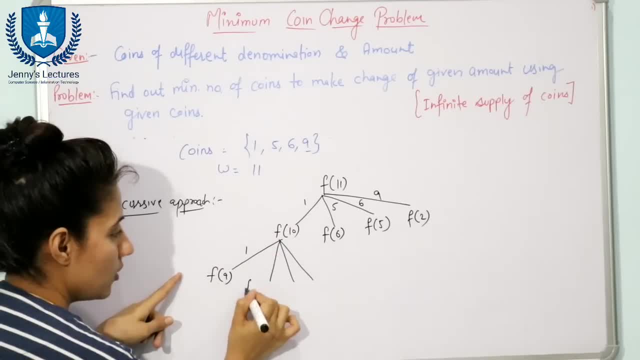 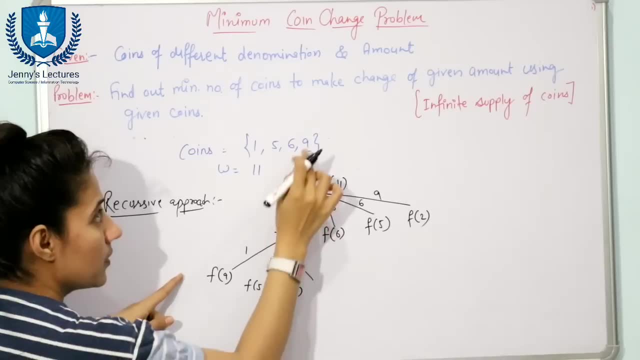 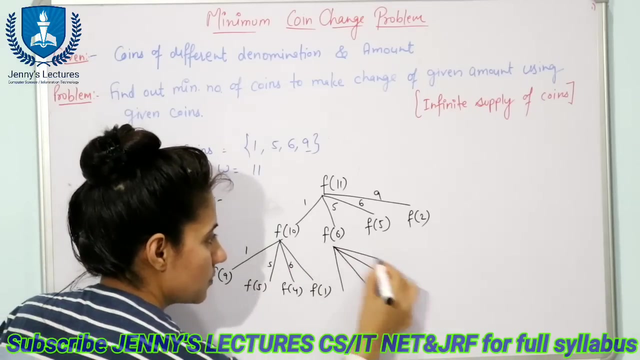 one, so the remaining amount would be 9. if you choose 5, remaining amount would be 10 minus 5, 5. if you choose the 6, then remaining amount would be 4, and if you choose 9, then remaining amount would be 1. same here you will have four choices: 1, then remaining is 5. if you choose 5, then remaining. 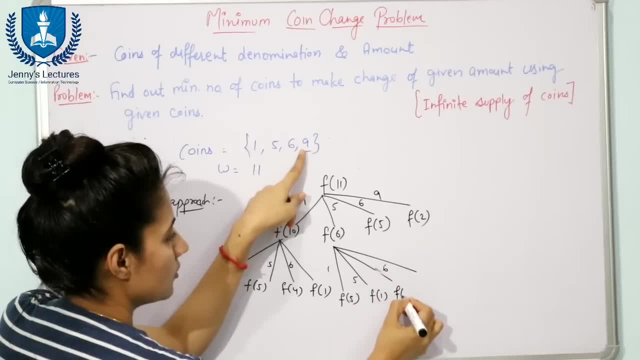 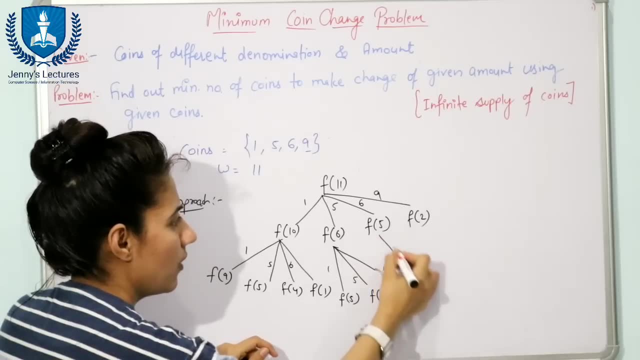 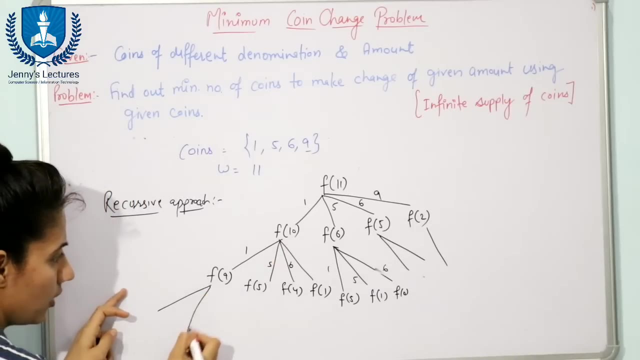 is 1. if you choose 6, then remaining is 0. sorry, here we have only three choices. we cannot choose this. 9 and like this. here also, you are having two choices. here you have one choice. now, if you go this this way, then here also we have four choices. and like this: 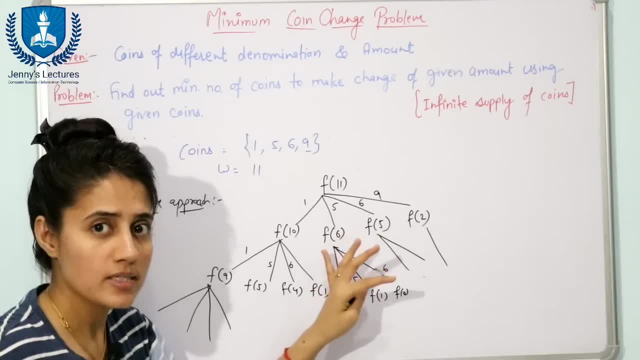 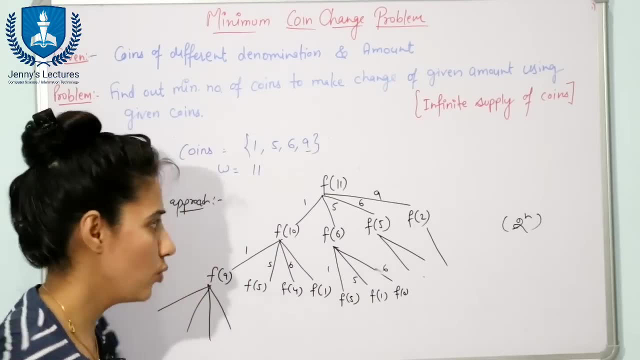 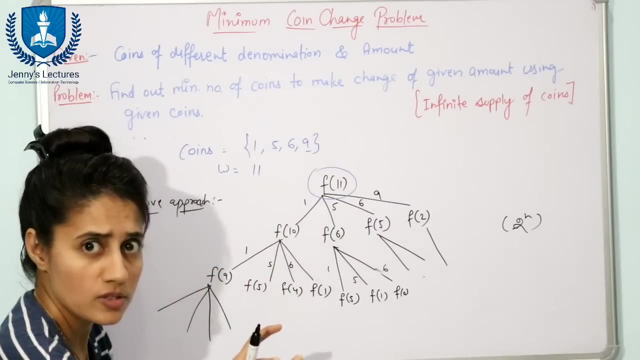 the question tree would be generated. now, what is the problem in this case? see here the time. complexity would be 2 raised to power, n exponential to solve this problem. and why so? see here here this. this complex problem is divided into sub problems. obviously, yes, this, see f5 here also. 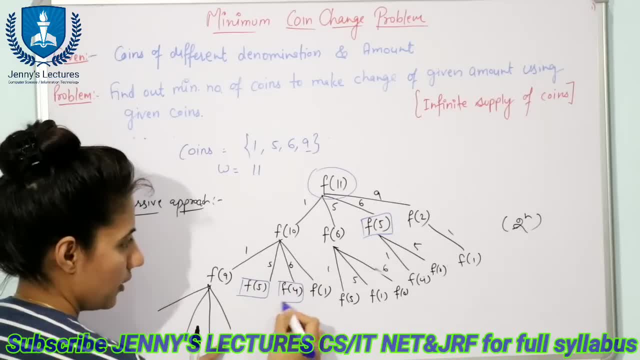 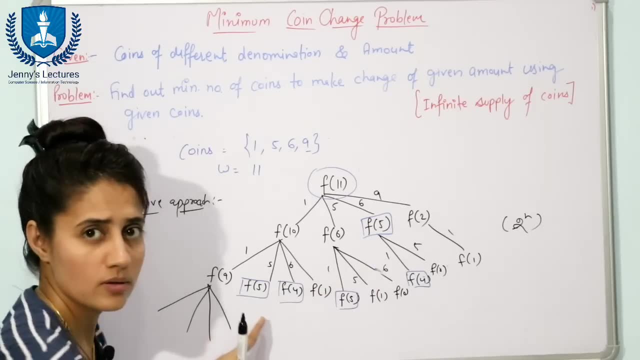 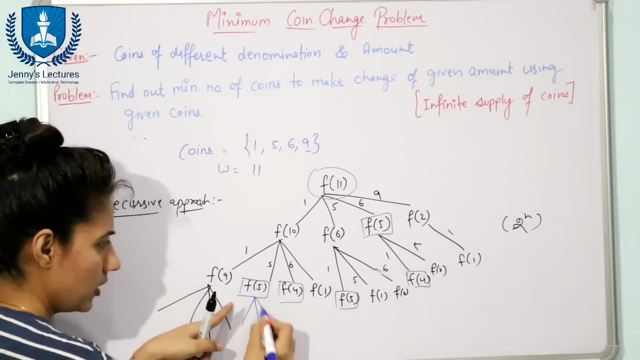 we are using 5 and see, here we are using f4, here also we are using f4. here also we are using f5. so this is what overlapping sub problems. but in case of recursion, when you are using this, here also we will compute this recursion tree and when we will call this f5. 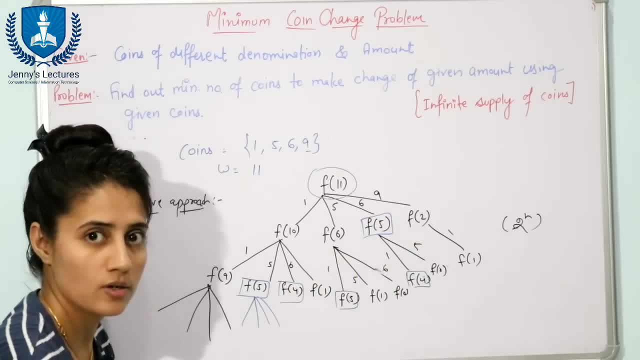 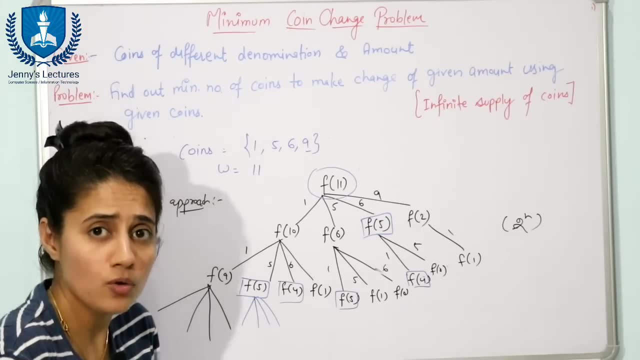 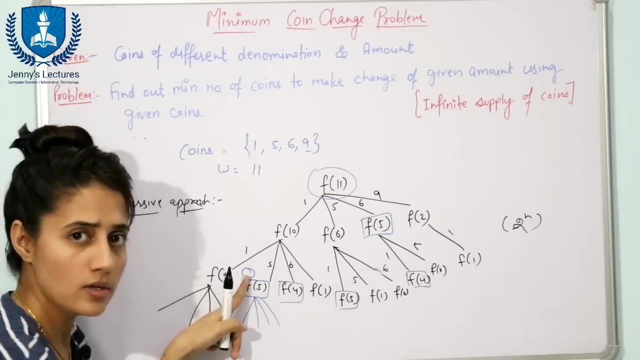 again. then again this recursion tree would be generated. so these sub problems are computed again and again, or you can say recomputed. so that is wastage of time. now what we can do if we solve this problem, okay and so. so we got some result, so we can store that result and after that in future sometimes we got this call f of i. then 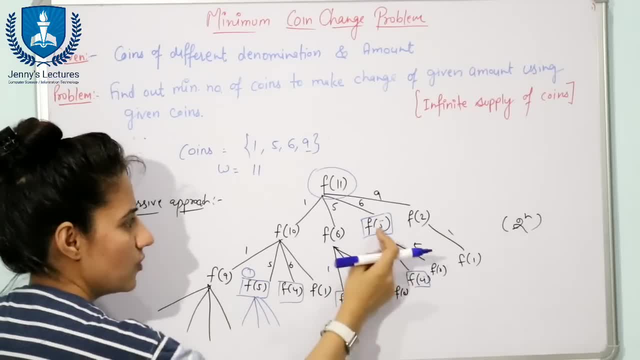 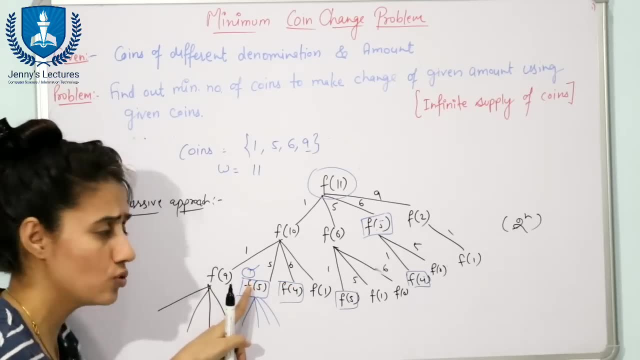 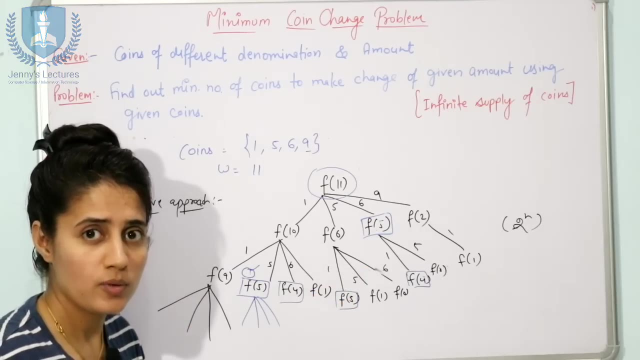 rather than generating, or rather than calling this function, rather than generating this recursive tree, for this one, we, we just choose this value. now, we just take this value because we have already stored this value. so that is something known as dynamic programming, and in that case, obviously, time comes in time, complexity would be decreased because number of computations would be decreased. 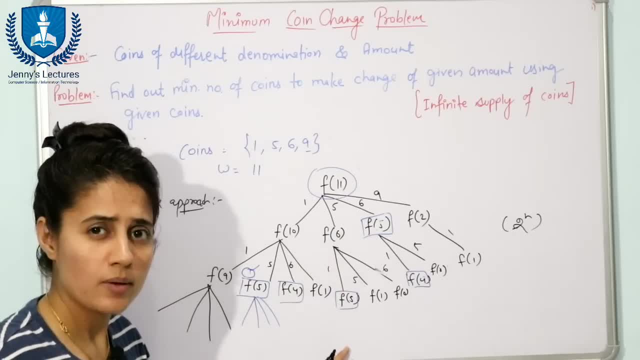 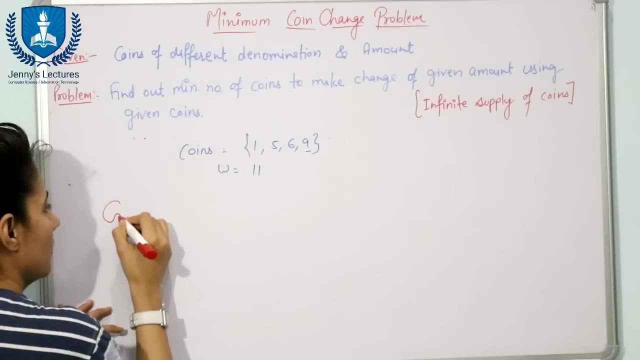 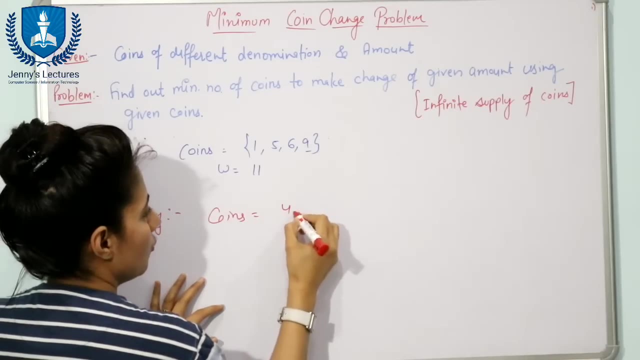 so that is why we are not using recursion here. what is the difference between recursion and dynamic programming? that i have explained very clearly in that previous video. so now, one more drawback of greedy algorithm is: see, suppose i am taking one more example here. coins are 4, 10 and 25 and amount given is 41. 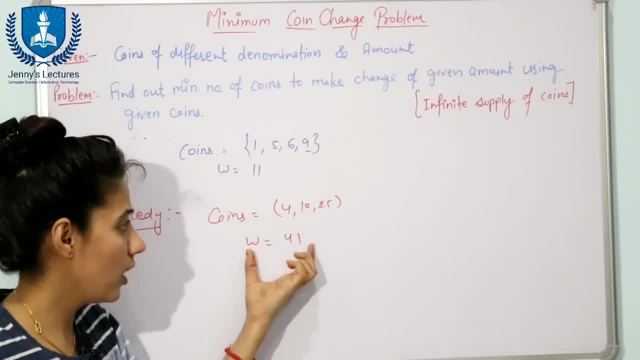 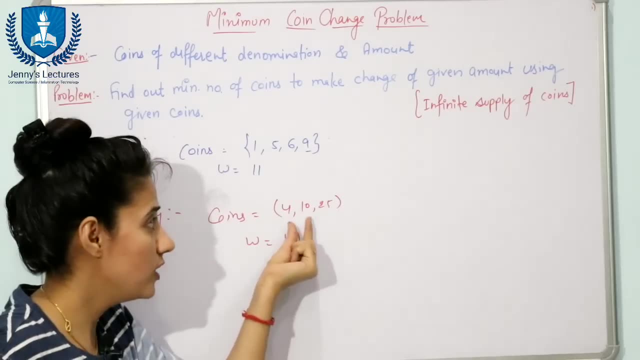 now you have to apply here, you have to solve this problem and you have to find out minimum number of make this sum, to make this sum using these number of coins, coins of these denominations. fine, and you have, we have infinite supply of coins. then, according to greedy method, what you will do first, 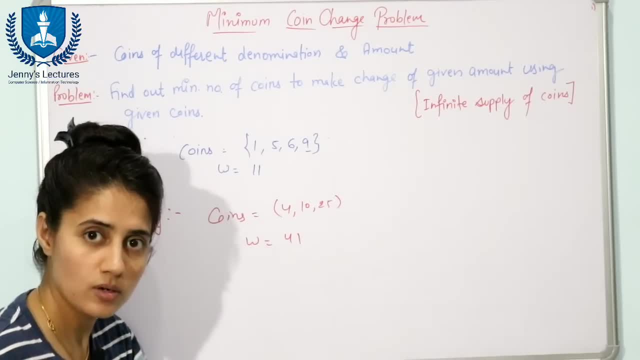 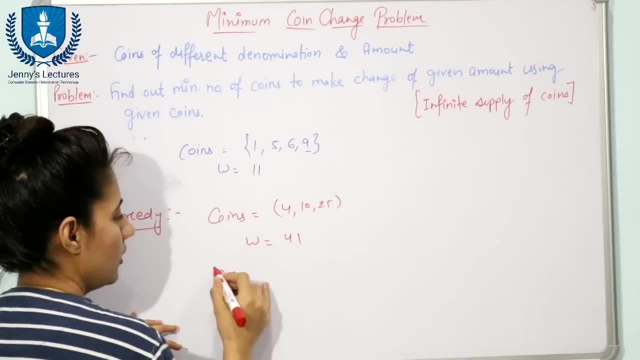 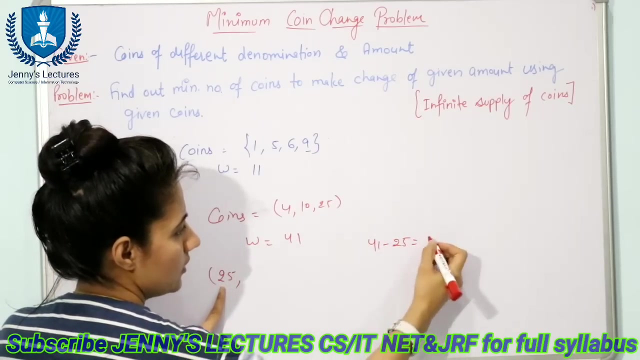 of all, the highest denomination coins should be chosen, but that should be obviously less than or equal to this sum. so what we can take is, first of all, we will take 25 now. after taking 25, the remaining amount is 41 minus 25. that is, i guess, 16. now for 16, which coin you will take we can take? 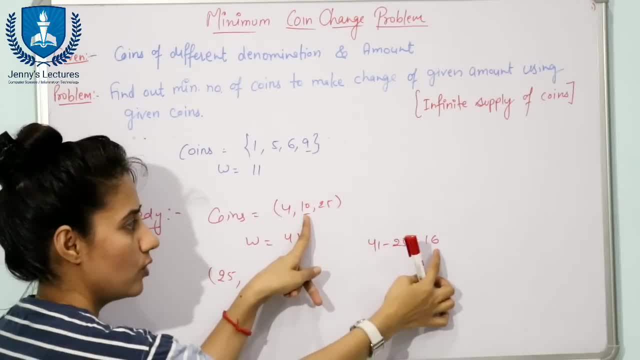 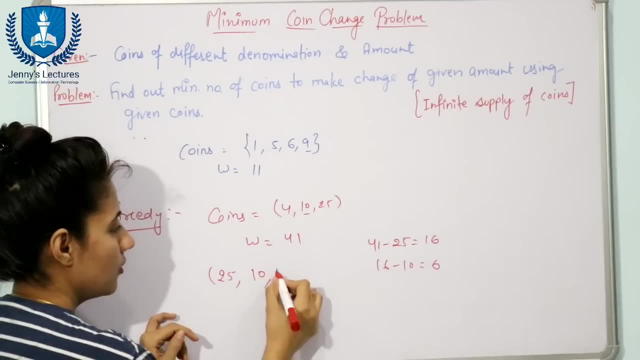 10, because highest is this one which is less than or equal to the 16, so we will take 10. now remaining is 16 minus 10 is 6. now for 6, you will take 4. remaining is 6 minus 4 is 2. but now you. 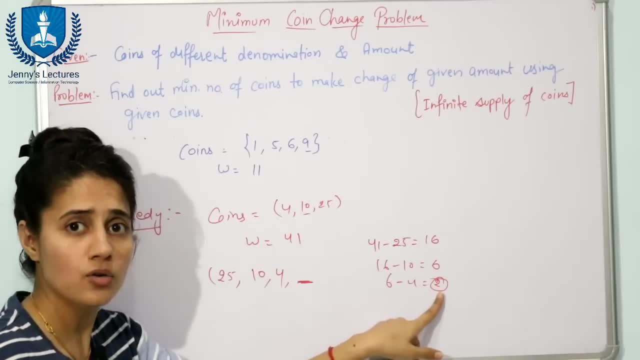 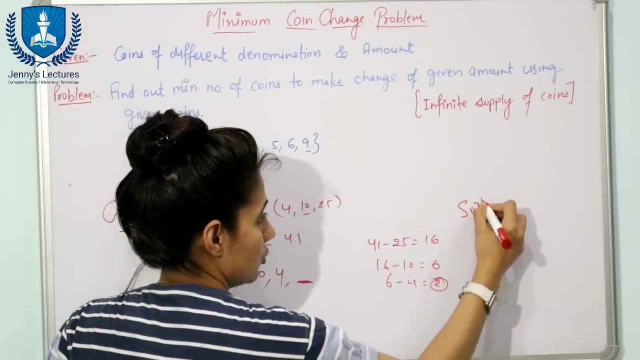 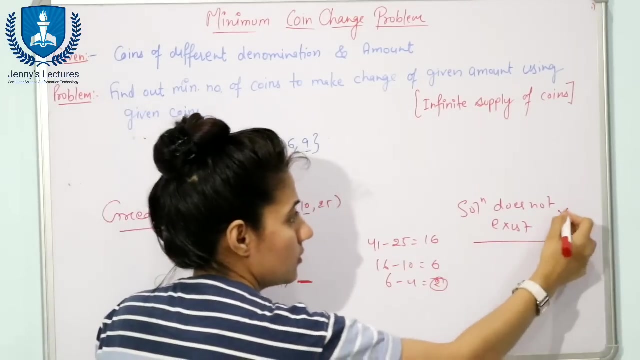 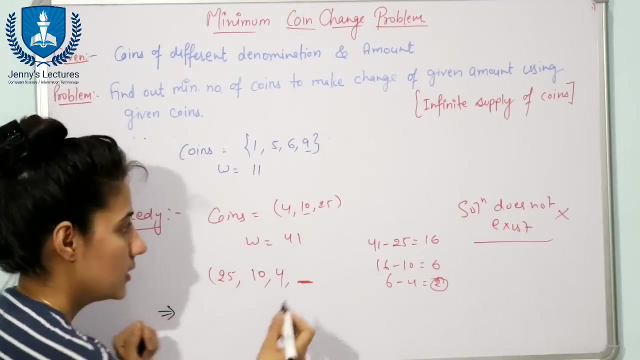 cannot choose any coin because we do not have any coin which is less than or equal to this 2. so according to greedy approach, solution does not exist. fine, but that is not the right answer. solution exists here. when you apply dynamic programming, then you will find the solution. now the solution is we can choose one 25 rupee coin and 4, 4, 4 and. 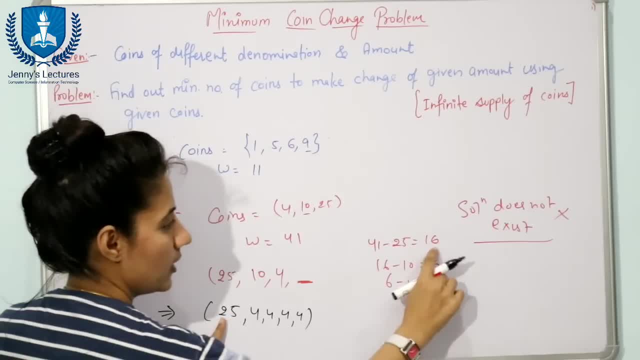 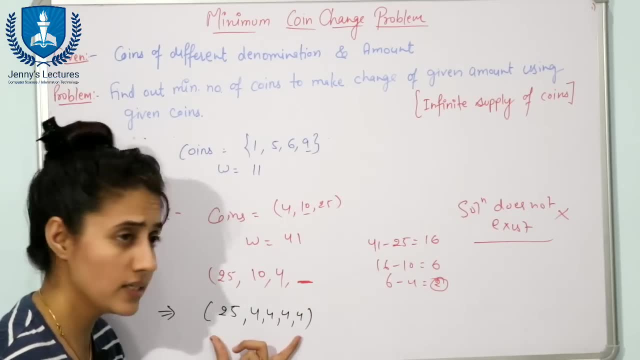 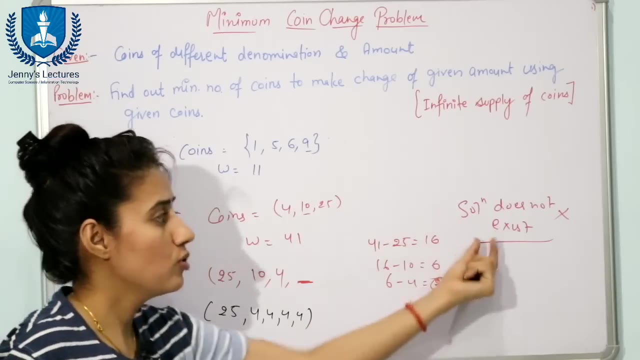 4, because after choosing this, 25 remaining is 16. so we can choose 4, 4 rupees coin, and that would make a sum of 41. so solution exists. number of coins needed are 1, 2, 3, 4, 5, but according to greedy algorithm, solution does not exist. so this is another drawback of this. 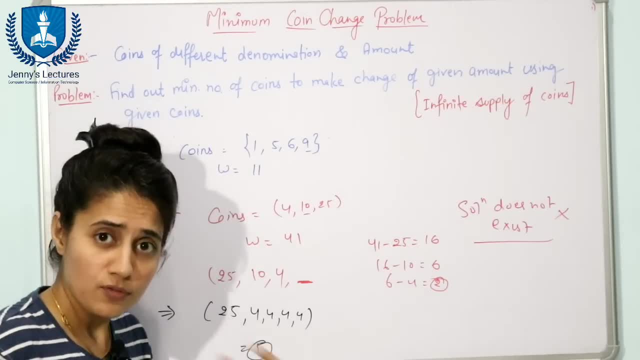 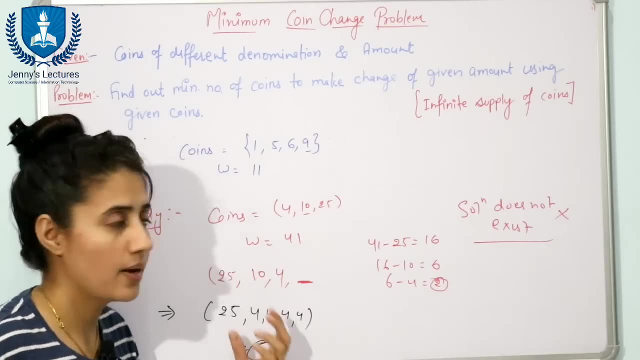 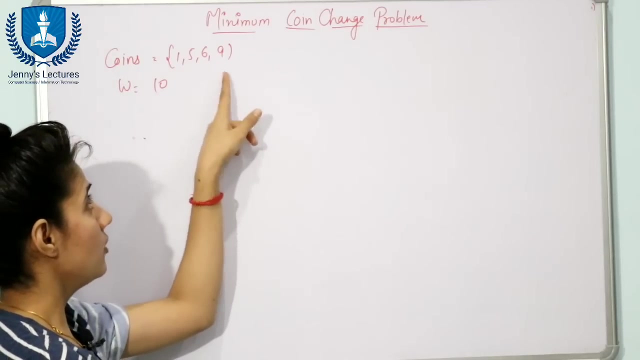 greedy algorithm. sometimes it does not work, but if solution exists, then dynamic programming will always give you the solution, the optimal solution. now let us take one example and we will apply dynamic programming to solve that thing. so the question is: you are given coins of different denominations- 1, 5, 6 and 9- and the amount given is 10.. now you have to find out the minimum number of. 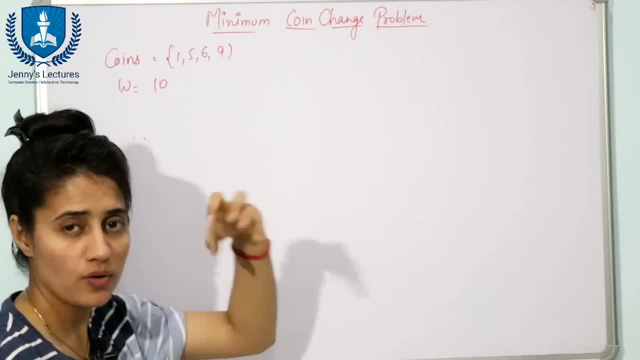 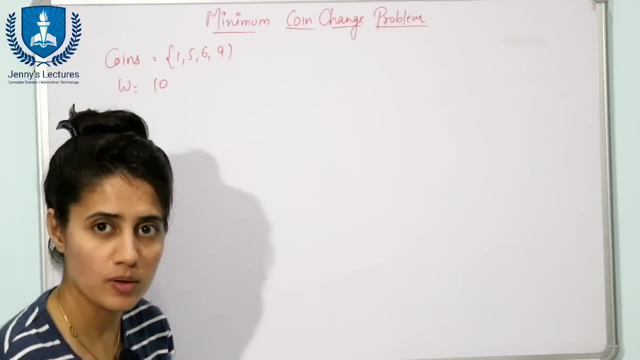 coins needed to make this sum. you have infinite supply of coins. now we are using dynamic programming approach, so we will divide this complex problem into simpler sub problems and we are using tabulation method. or you can say that bottom-up approach- fine, now how, how that complex problem will fall. cardboard method. or you can say that bottom-up approach, fine, now how, how? that a minimum number of coins needed to make this sum. now how, how that lever Project. well, so, from this article, if you actually used all of these terms, so after all of these terms, what do you use in your dynamic programming program? you will find this: 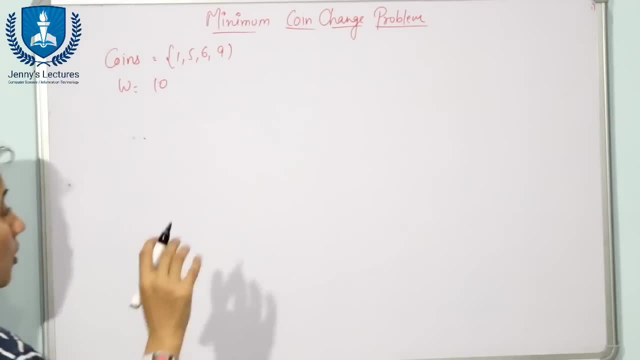 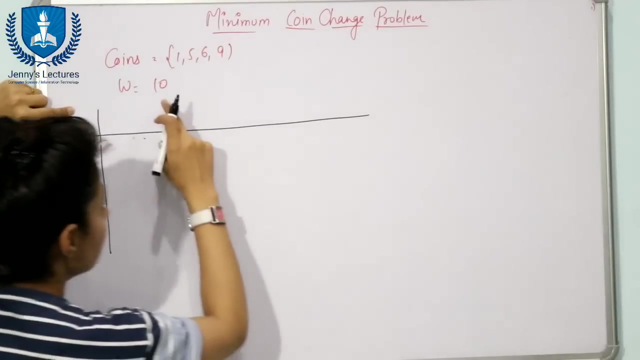 that bottom up approach. fine, now how, how that thing is, how this thing is to be solved. this side, to this side, we will take, you know, coins 1, 5, 6 and 9. we will draw a table and this side, we are going to take this amount. so we are going to divide this problem into simpler problems. 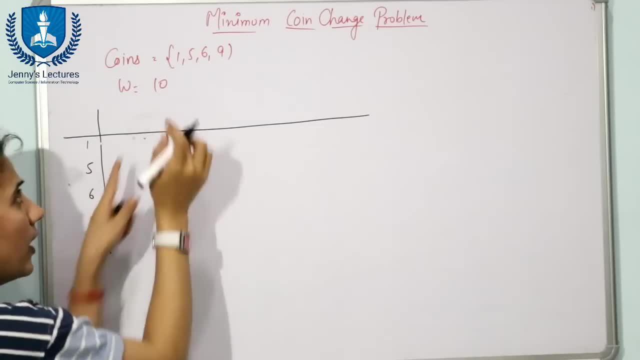 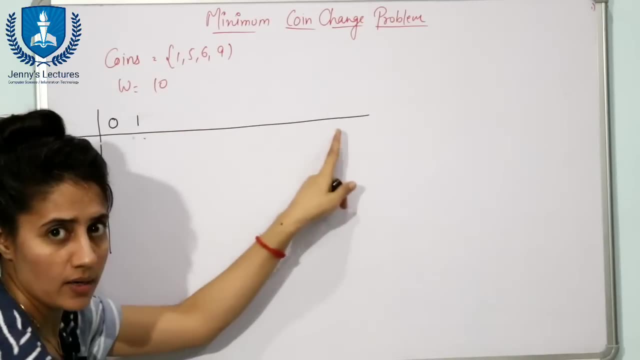 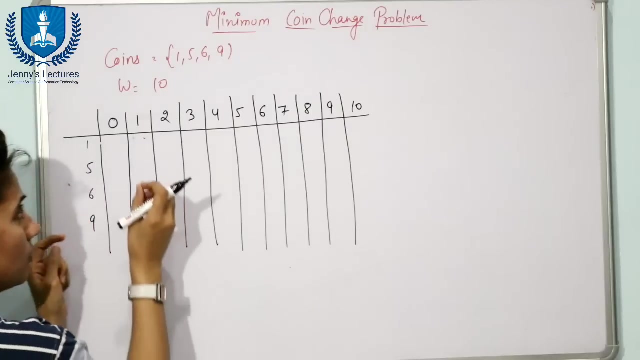 so we are not going to write here 10, simply we will divide this. so we will start from 0 and then from 0 to 10. we will write here: okay, so we have divided this into sub problems and we will solve, we will. we will, you know, compute these sub problems and we will store the result. 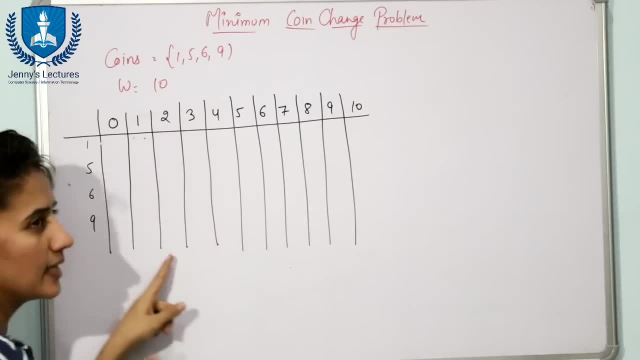 of these sub problems into these rows. or you can say cells: okay, now how to find out. this side we have coins and this side we have amount. or you can say we are going to take two variables: i- this, this side, and j- this side. we are going to apply the four loops when you are, you are going to code. 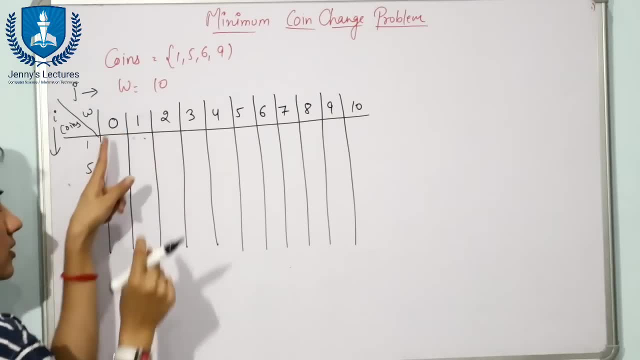 this. okay. now see when the sum is zero and at starting i is, i is from zero, one, two, three, like this, i will increase. so when i zero, then we have only coin of denomination one and sum is what- zero. so how many minimum number of coins you need to make this sum? see if i ask you the total number. 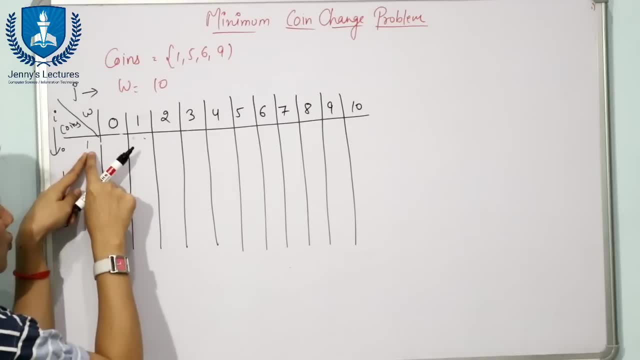 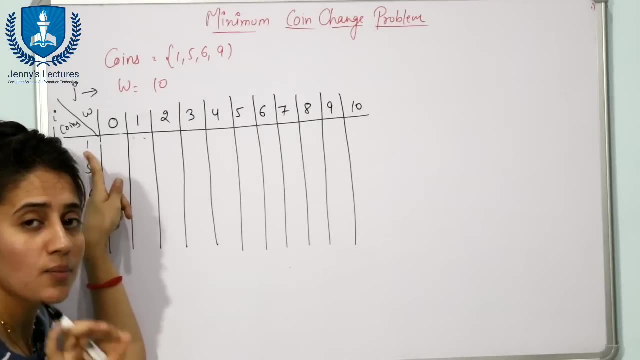 of ways, then you can say one how. if we do not choose this coin, then obviously you will make a sum of zero. so that is why you say you can say that one way is there, but here i am asking the minimum number of coins. if you do not choose any coin, then minimum number of coins are zero. 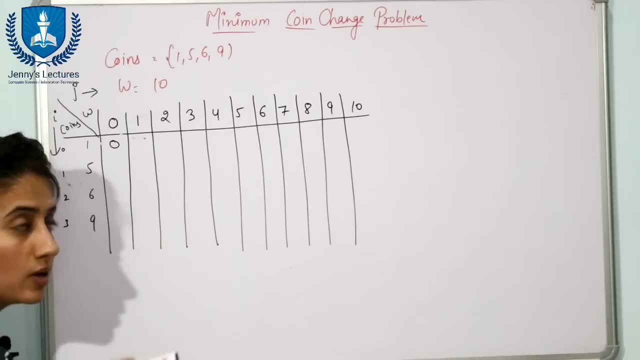 so here you will write what? zero. so in this column, where the amount is zero, we will write zero, zero, zero and zero. because we are not choosing any. we are not choosing any coin, so that is why the number of coins we are choosing are zero. okay, now, if sum is. 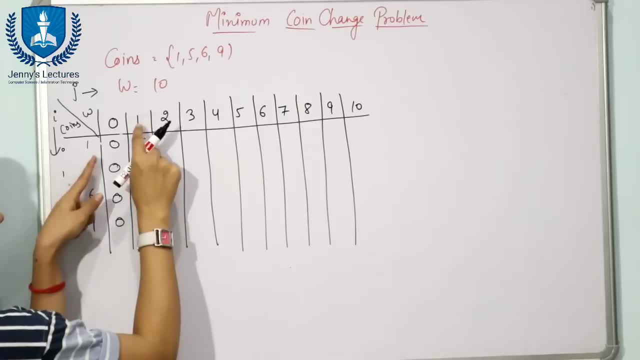 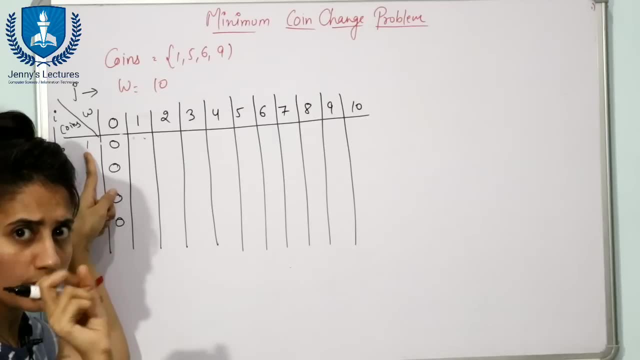 one. now check how to solve this. if sum is one, and we are have, we are having only coin of denomination one, we have only one, one rupee coin. then how many coins you need to make this sum? one coin. if the sum is two, you have to make this sum, you have to make this amount two and you have only coin of denomination. 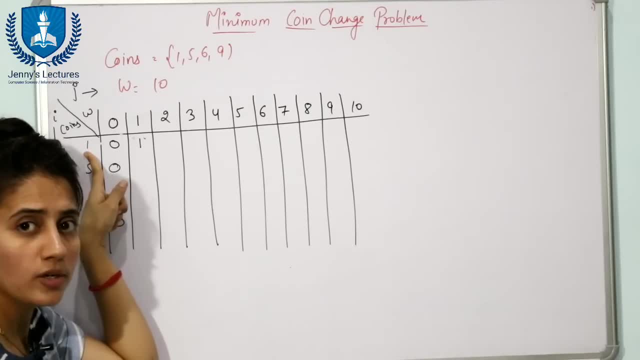 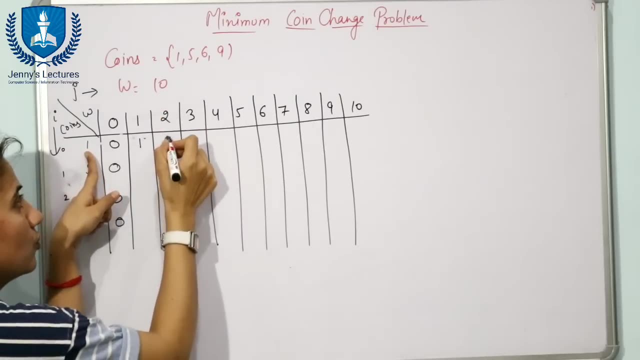 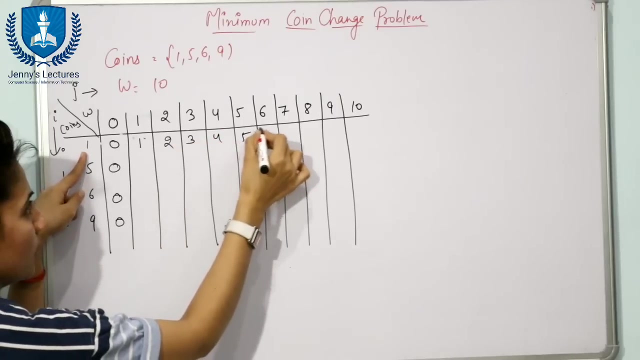 one. then you how many coins? you need two coins you need, okay, two, one rupee coin. that is why i can say you can make a sum of two, two to make amount of three how many one rupee coin you need, because you have only one rupee coin. three here, four here, five, six, seven, eight, nine and ten, like this: 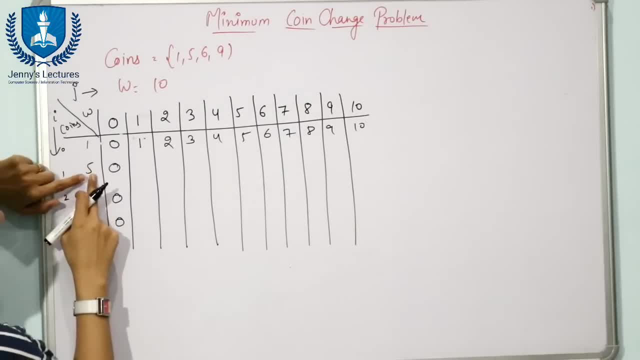 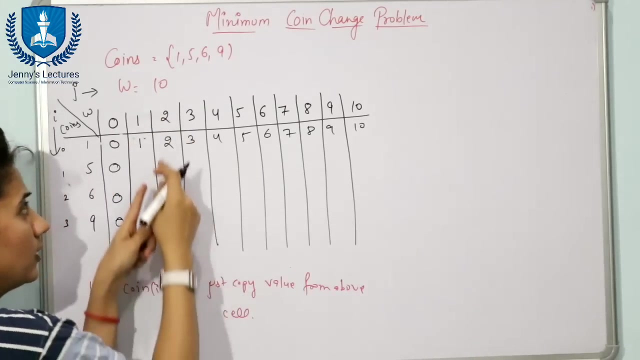 fine, now i value has been increased. ok, now we have coins of denomination one and five. now check, see, the simple rule is here also. the simple rule is: if this coin value is greater than this- this amount value, or you can say this j value- then just copy the value from the above Excel. this is: 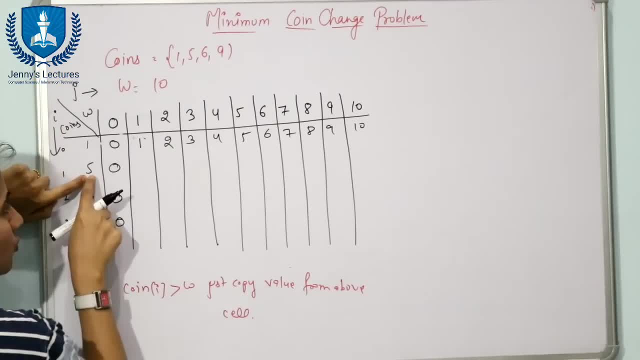 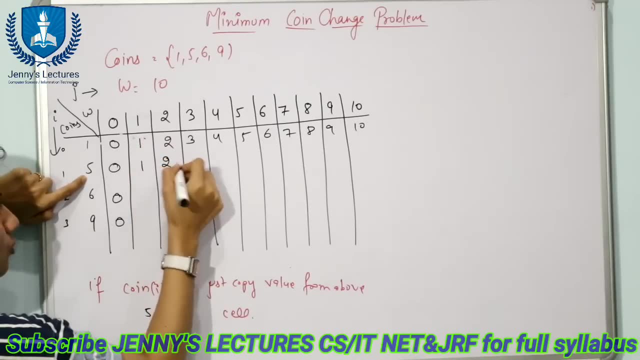 the simple trick. okay, now see this. this coin value is five and one, so five is equal to. so this five is greater than this one. so simply, we will write value from above cell. here also two, here also three, here also four. now the coin value is five, here also five. so this condition is not. 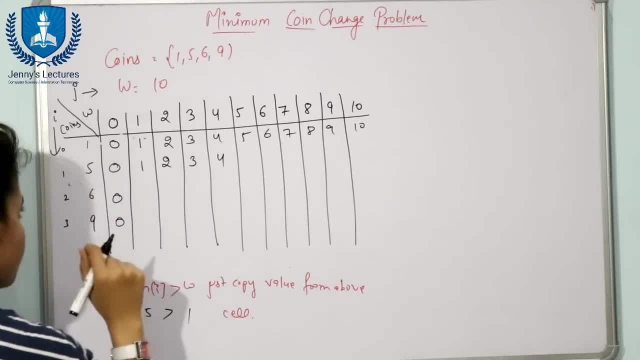 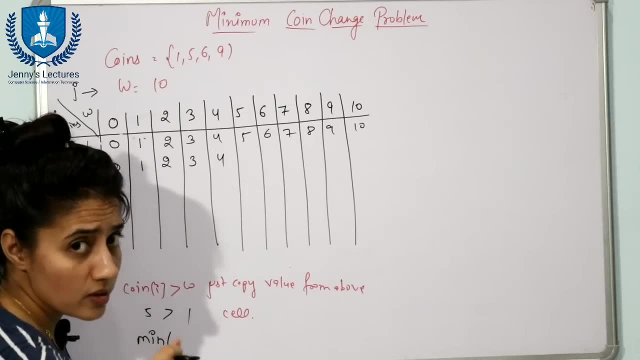 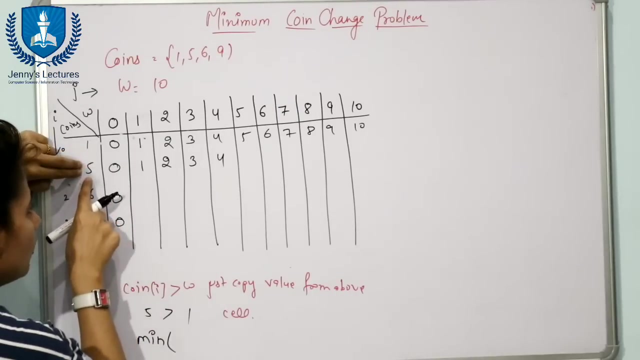 true. now you have to do what now? how to choose. now suppose you have to select something minimum, because we are choosing, we are, we are going to find minimum number of coins, so we are going to select minimum, out of which we are choosing minimum. see, if we do not choose this coin, then 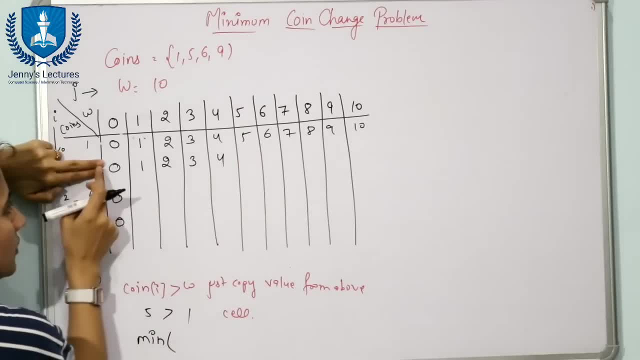 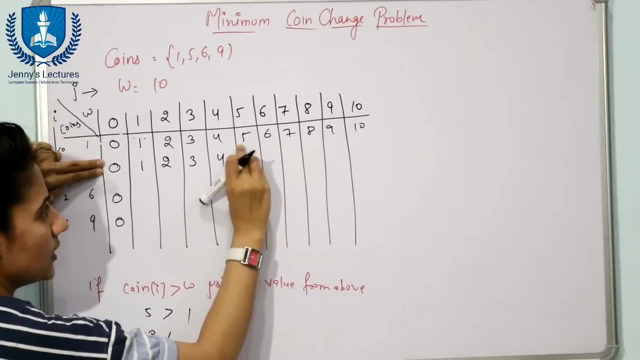 how? in how many ways you can make a sum of five, because if you do not choose this one, then you have only coin of denomination one, and then the minimum number of coins needed are five. okay, simply the take the value from the above cell or, if we choose, if we select this coin. 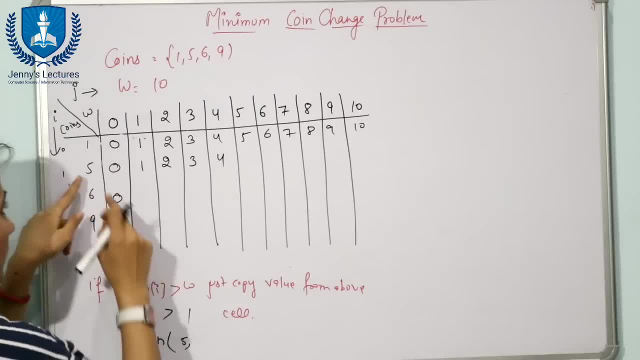 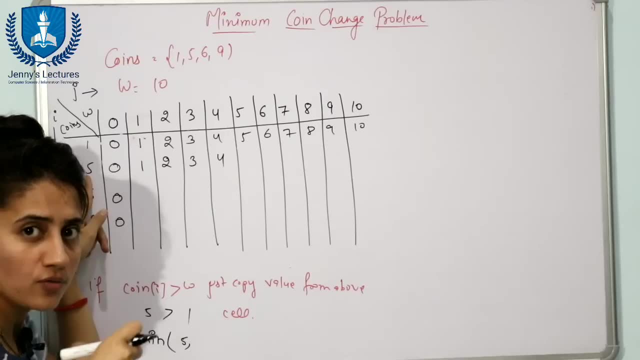 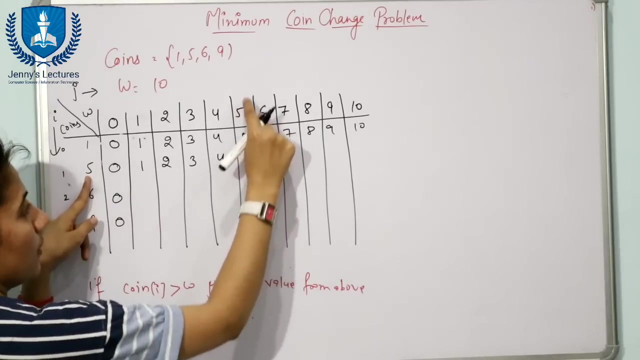 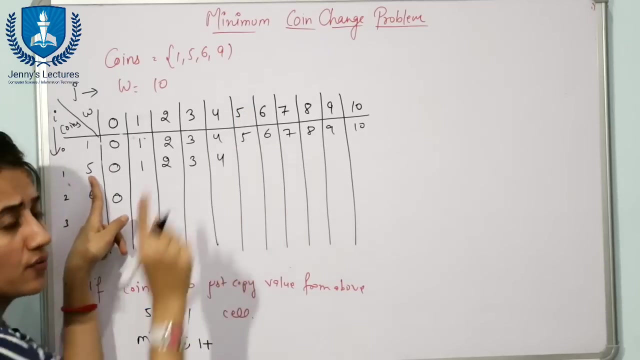 then how many coins you need if we choose this coin, if we are choosing this one means we have. we have taken one coin of five rupee, so here we will take one plus, okay, plus see, the amount is five. if you have taken one five rupee coin, then amount remaining is this: five minus this value. five minus five is zero, so in 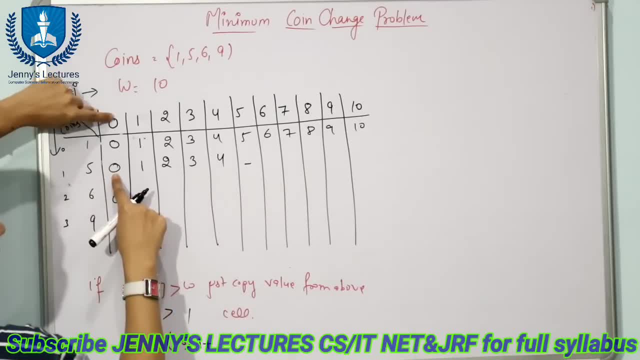 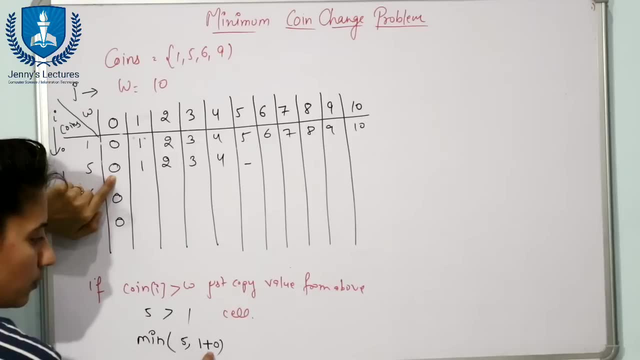 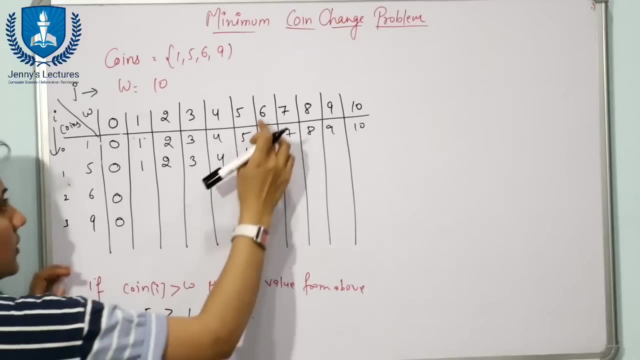 this in this same row. we are going to a column having the amount zero. now here we have. the value is zero, one plus zero. so minimum of five and one plus zero is one, that is one. so here we will, here we will write what one same for this one. see if it. if you do not choose this five coin, then 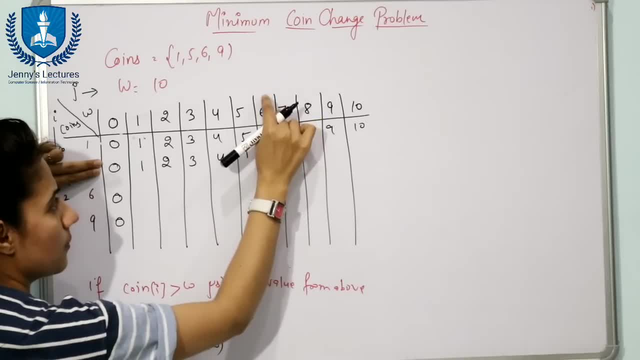 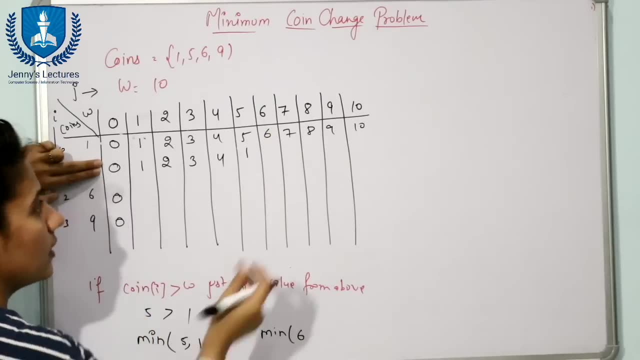 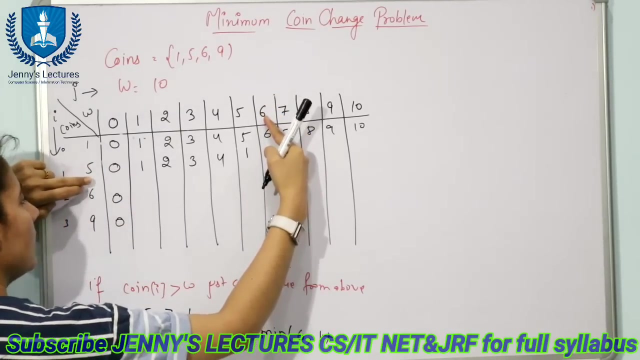 how many minimum number of coins you need to make this sum: six coin minimum of six. just see the value of the above cell. fine, and if you select this coin, if you select this coin, then one coin you have already selected, you have already taken. so one plus now amount is six. you have to make this amount and we have chosen one five rupee coin. 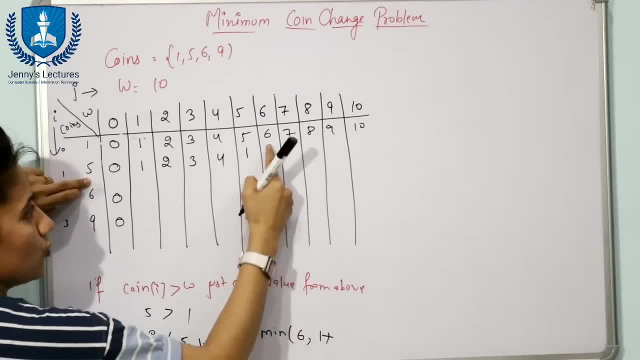 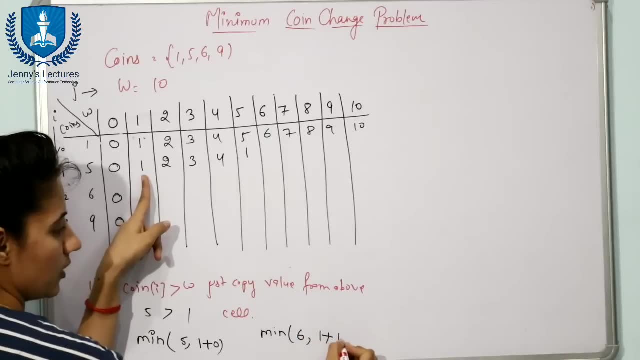 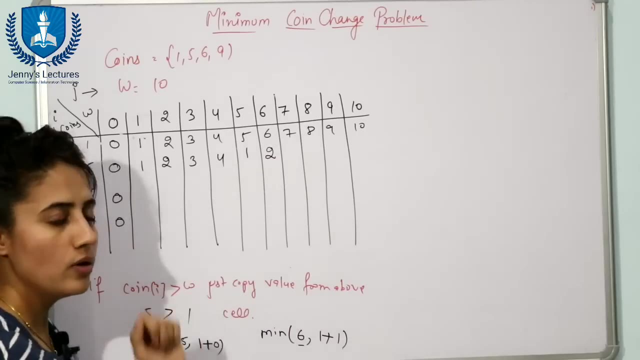 so remaining amount is six minus five, that is one. so in the same row you will go the column having amount, having amount value one. so here we have one. so just add one here now. minimum of six and two, which one is minimum two. so here we will take what two same. for this one we will take minimum of. 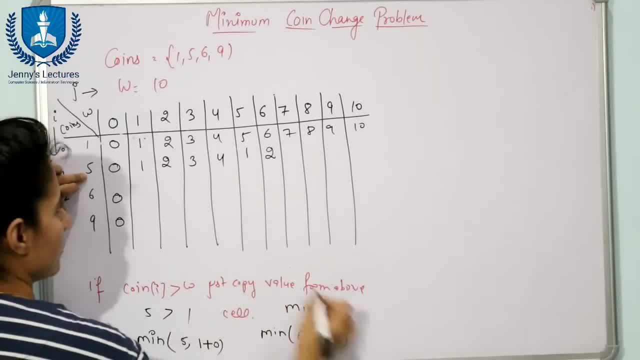 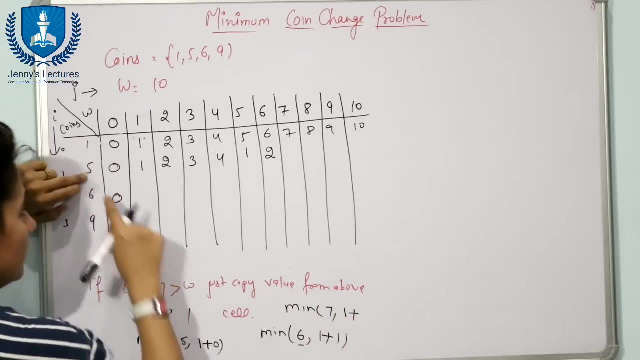 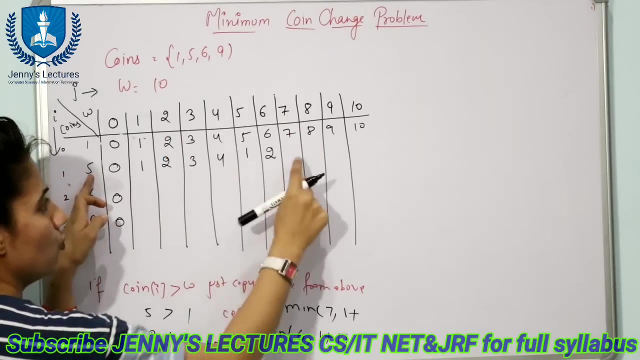 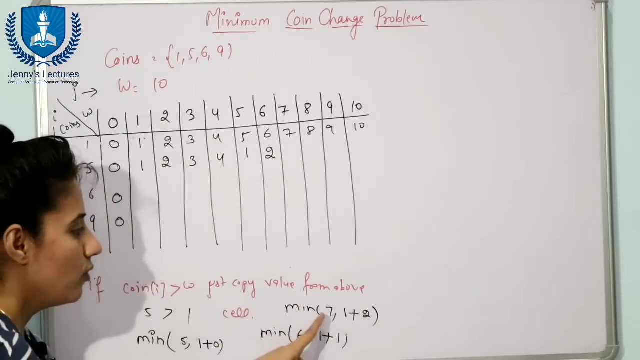 this value seven and if you choose this five, then we have taken one coin of this denomination plus. remaining amount is seven minus five, that is two. now check how many coins you need to make amount two. now in the same row you'll to a column having amount two, two points. you need two. so minimum of seven and three is three. 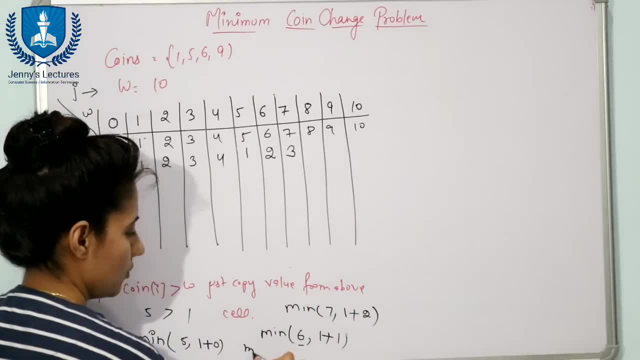 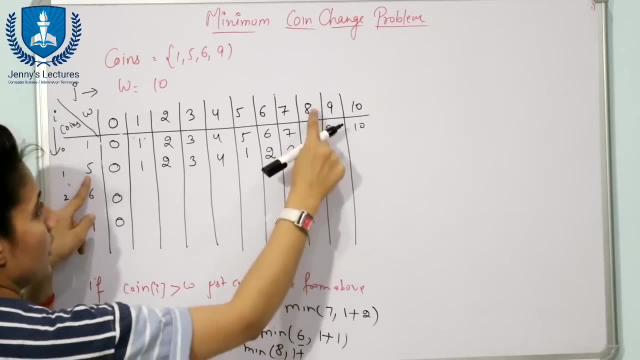 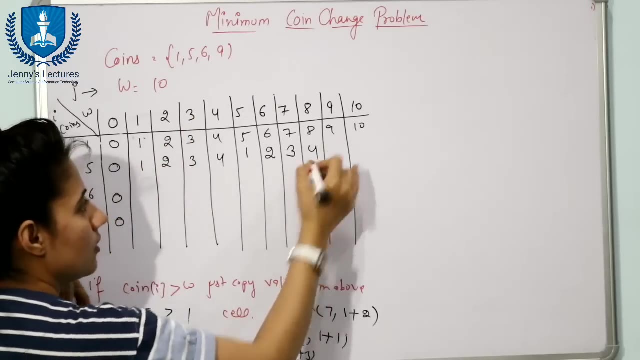 same with eight. you will take what? what? minimum of eight comma. eight minus five is three. one plus eight minus five is three. this column is three, having some one plus three. minimum of eight and four. we will take four. same with this one here. minimum of this, minimum of this. 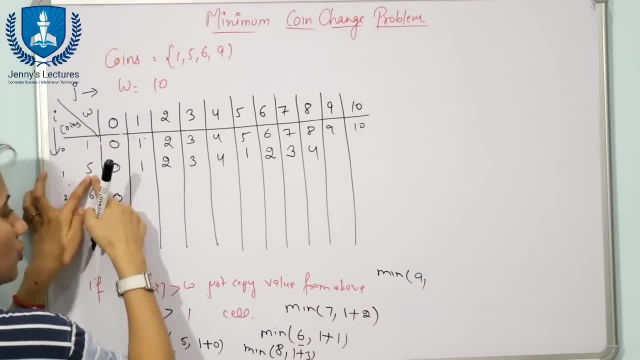 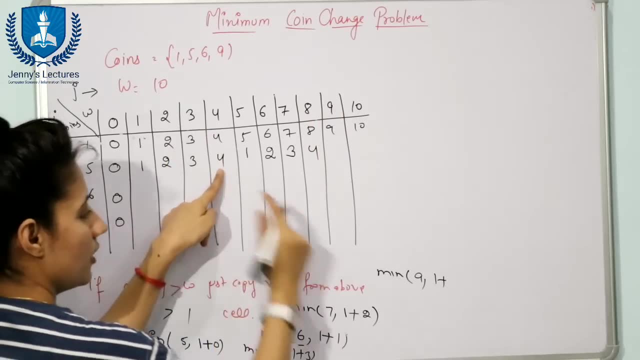 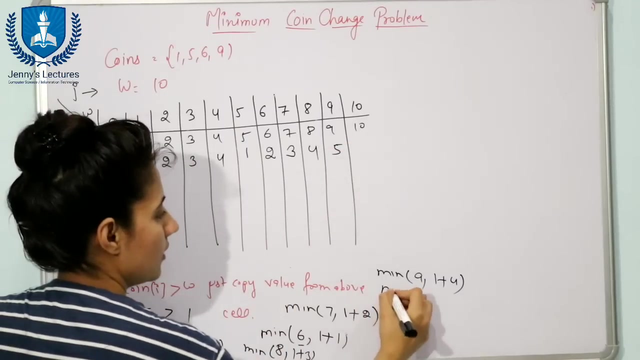 above value nine without using this five. if we choose this five, then one plus remaining amount is nine minus five is four. now we'll go to the column having some four and four, then nine and five. here you will take what five? here you will take next, minimum of ten. 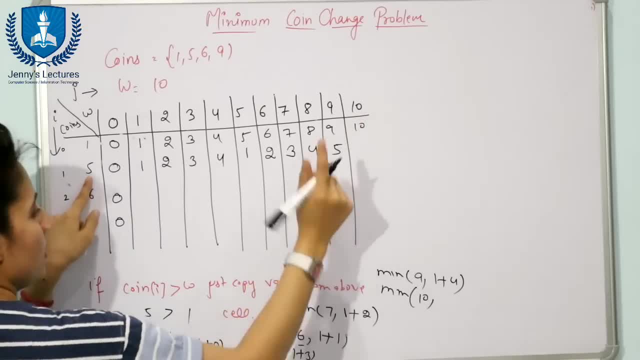 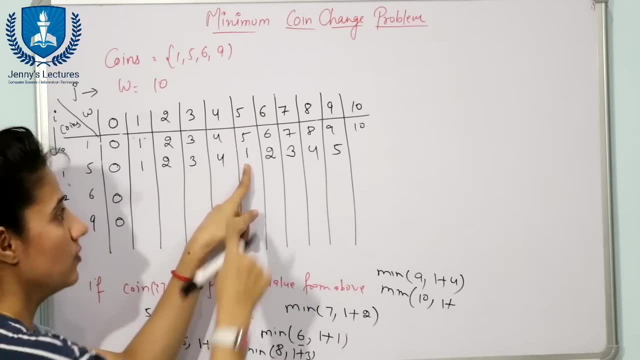 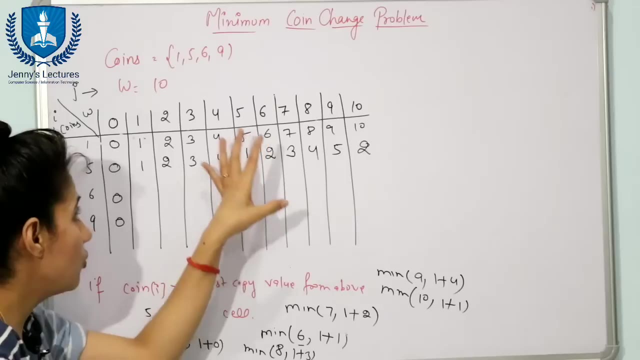 comma ten. comma ten minus five is five. so one plus ten minus five is five. go to this in this same row, go to the column having some five. here we have value one, so ten and two. the minimum is what? two? so this is how you are going to fill this table, the formula i will write in the end. so i guess. 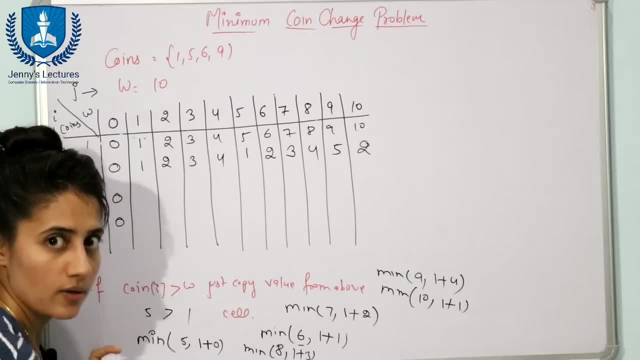 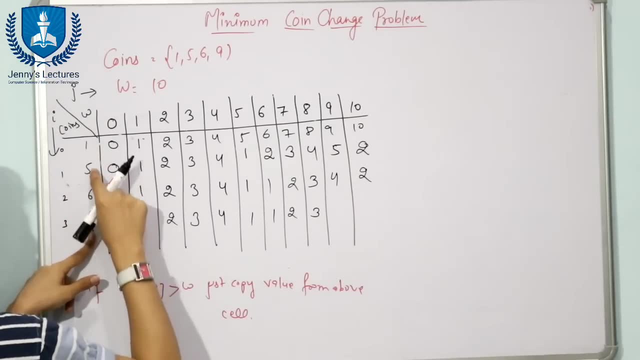 you can fill this table now. i am just going to write the values here now. finally, uh, check for these values. see, we have now i value is 3. now we have coins of denomination 1, 5, 6 and 9, so till 0 to 8. we will copy the value from the above cell because 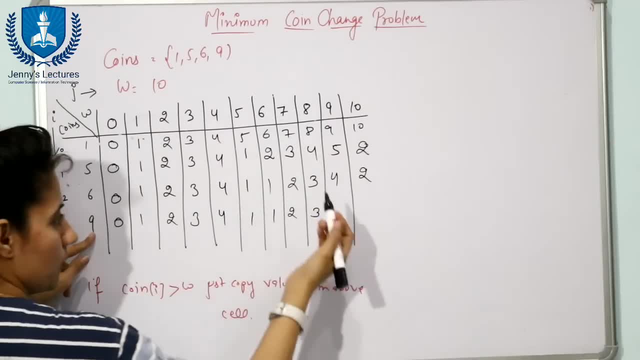 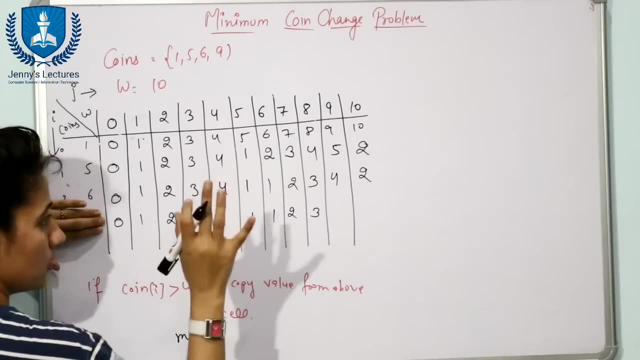 this value is greater than this one now at 9. what you will do? you will choose either this 4 minimum of see. if you will not choose this coin, then how? in how many ways? or you can say sorry, the minimum number of coins needed to make this sum using coins of these denomination, that is. 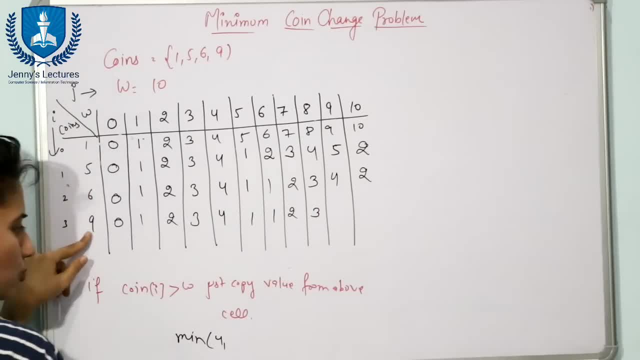 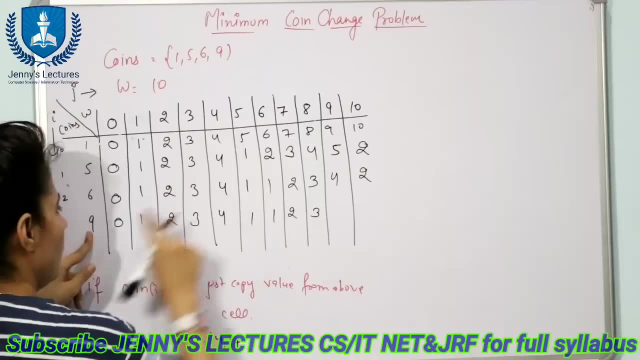 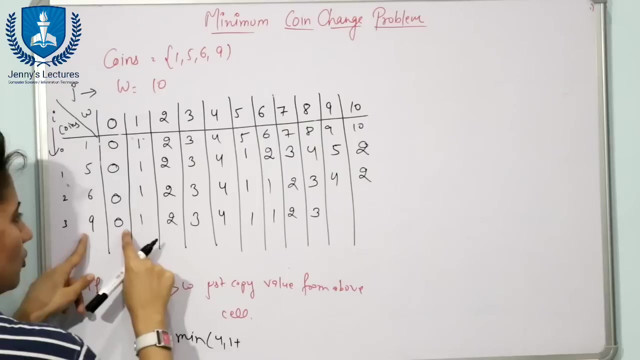 4, only so minimum of 4 comma. if you choose this one, then we have already chosen this 9. that is, you can say 1 coin, 1 plus. you have chosen this 9. amount is 9, so you have to reduce this value from this amount. 9 minus 9 is 0. in the same row, go to the column having value 0. 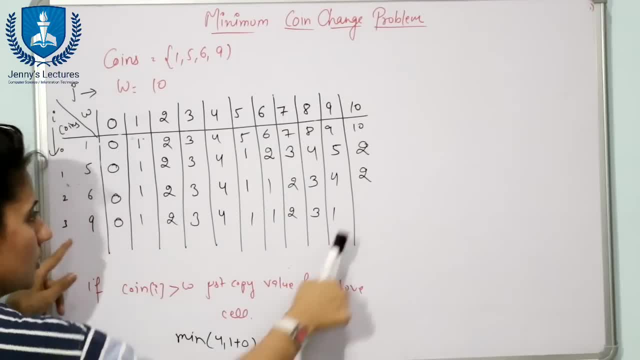 1 plus 0, 4 and 1. minimum is 1, same for this one, what you will choose. minimum of this: 2 and 1 plus 10 minus 9 is 1. so here you will go the same row, you will go the column having. 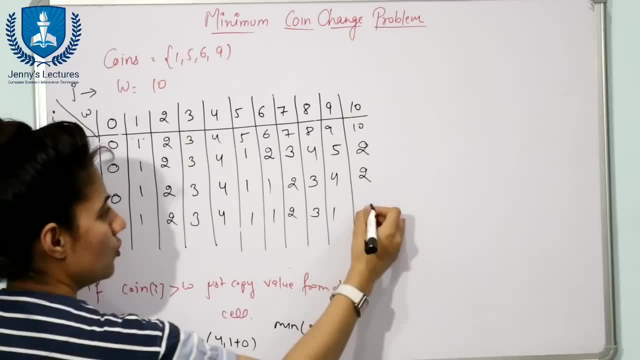 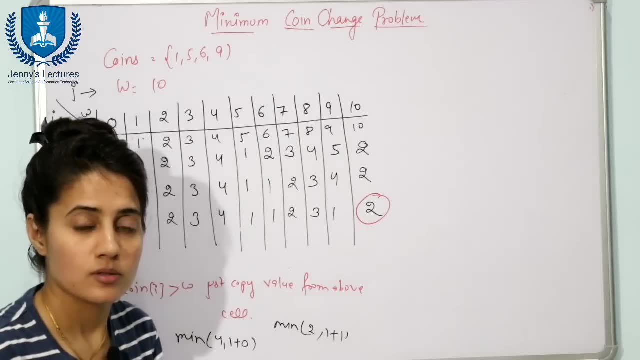 some 1, that is 1, 1 plus 1, 2. minimum of 2 and 2 is what? 2 only. so the answer is 2. the minimum number of coins needed to make this sum is 2. okay, and if you want to find out, see. 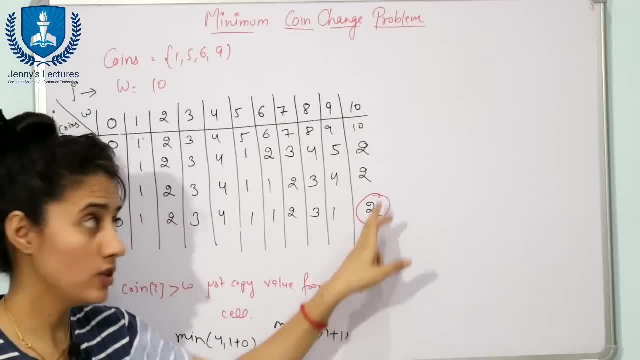 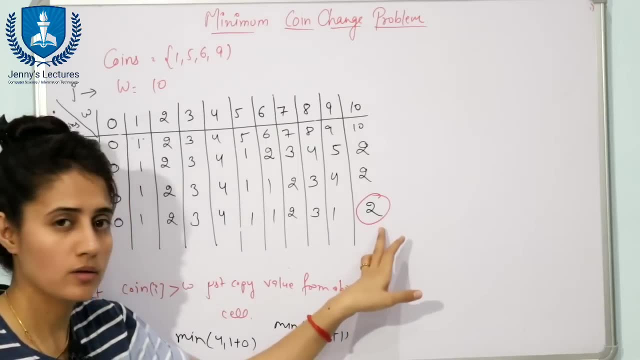 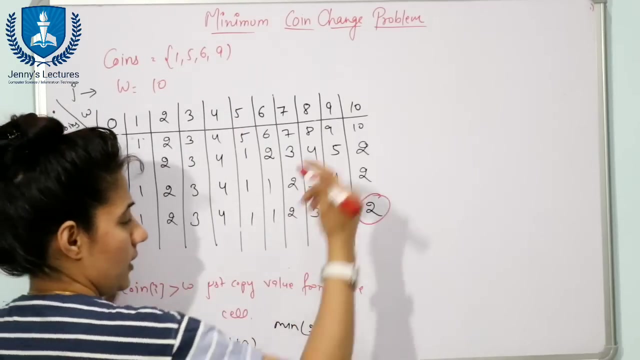 always, you will find the answer in this intersection of this last column and last row. and if you want to find out coins, of which denomination you are choosing, to find out the ceiling of ten, then how we will find out. see, now we are at here. only see, pointer is at. 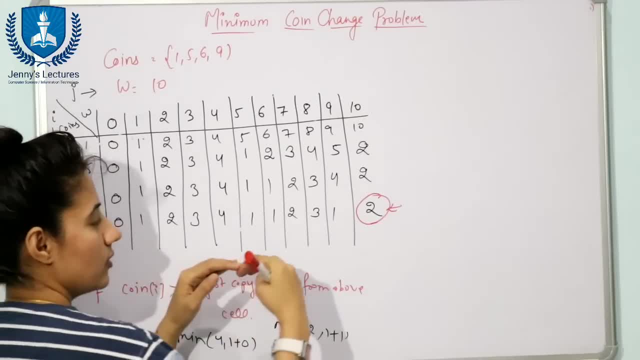 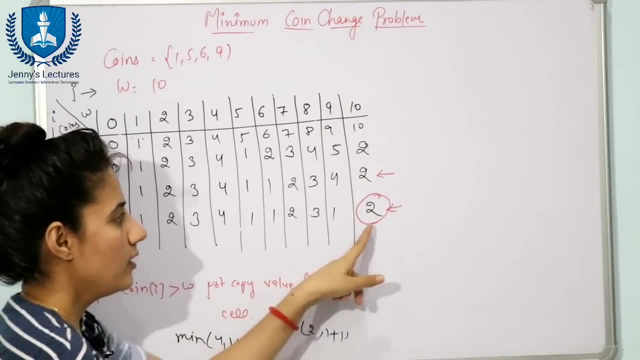 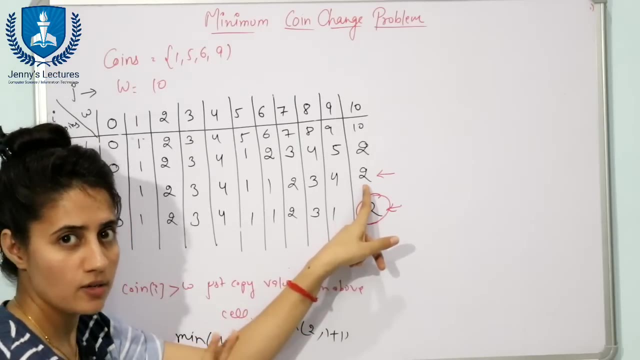 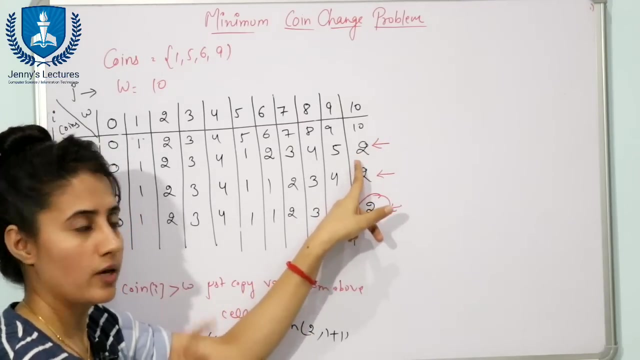 here only now. now the rule is what the? we will move the four, the pointer, one step backward here and you see the where. if the value is same which is here in this row, in this row, then then it is okay. then pointer will again move to upper row. here also we have two. here also we have two. then also, fine, we will not do, we will not do. 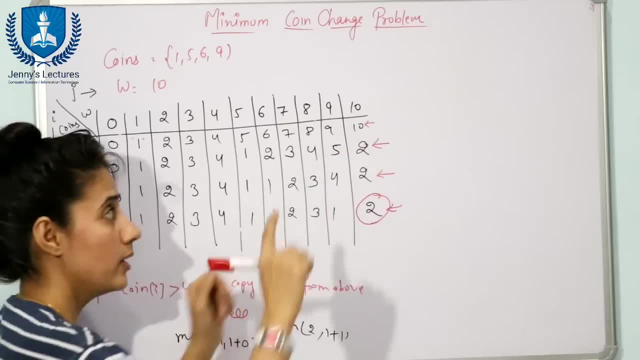 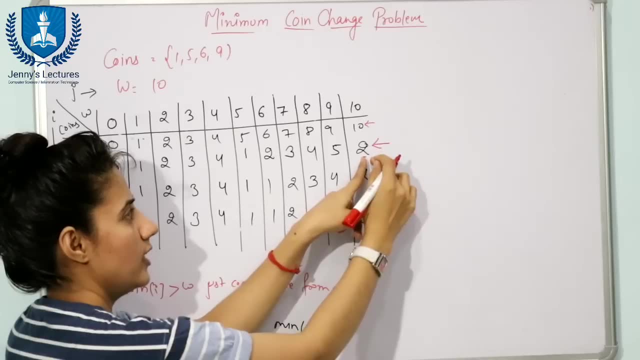 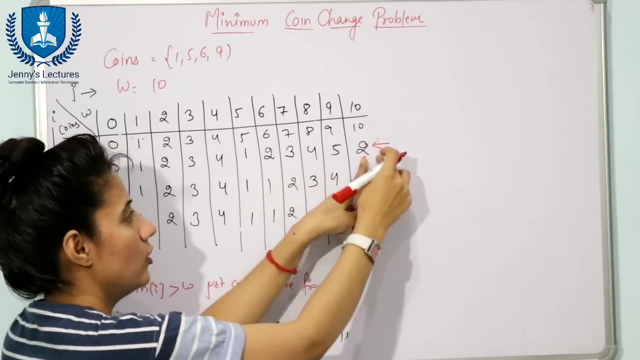 anything now we will move the pointer one step backward. now, see, the value has been changed. so it is for sure that this two, we are not getting this two from above, from this above cell, that is for sure. so now, now, what we will do, we will take so obviously, this two is we are getting this two. 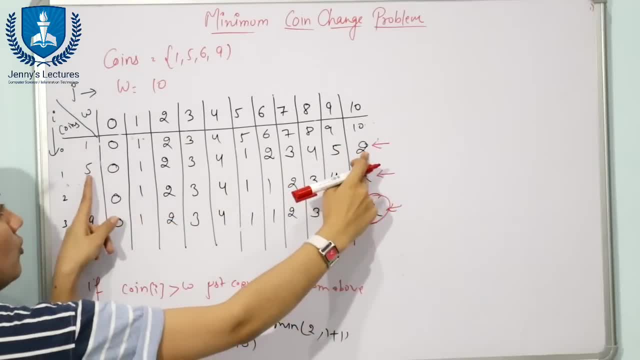 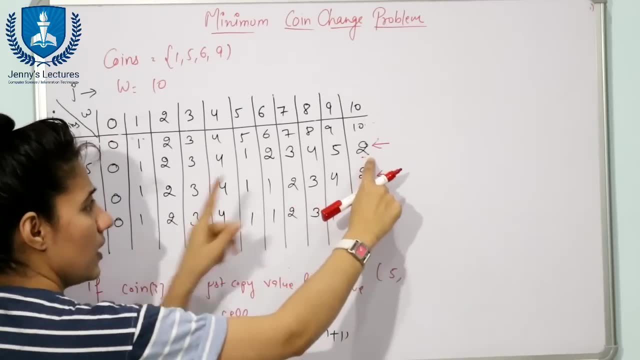 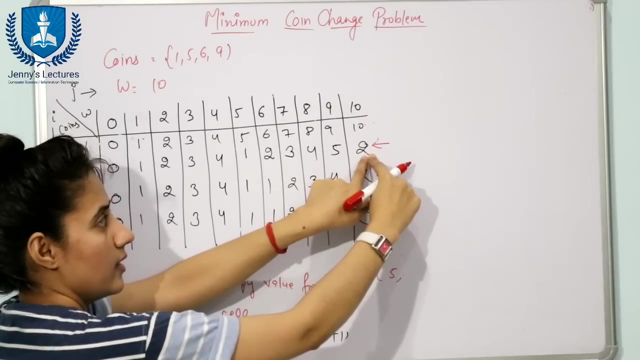 from this side only. so now we are going to take coin of this denomination that is five, so one coin we have taken now. what you have to do is now what you have to do is from this, from this amount, see because pointer at this side now, so in this column, what is the amount? 10, so from this amount. 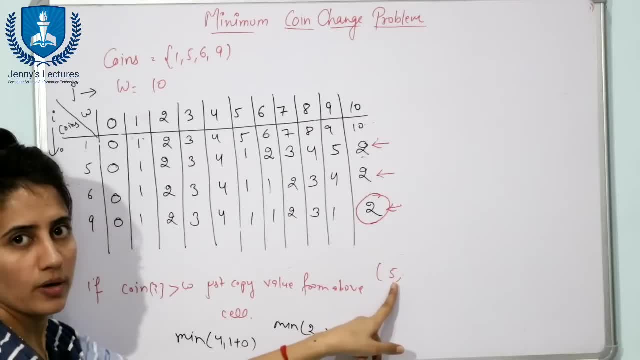 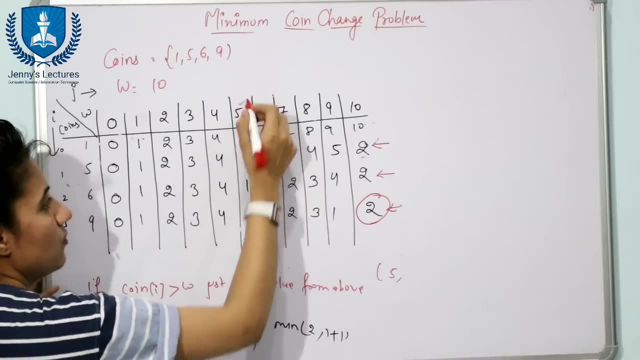 just reduce this value because we have taken this coin. so 10 minus 5 is 5. so in the same row, in this row, we have taken this value. so from this side only- so now we are going to take coin of this- you go to the column having some five. the pointer is now at one. okay, now same step would be applied. 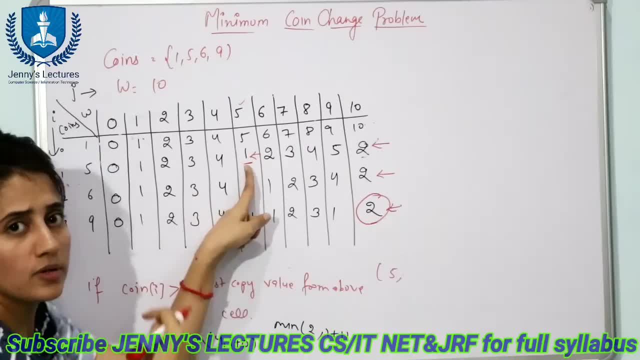 you have to choose this when value you are getting from this side or from upper cell. now check in the upper cell. the value is five. the value has been changed. so we are not getting this one from upper cell. we are getting this value from this side only. so again, you will choose five. 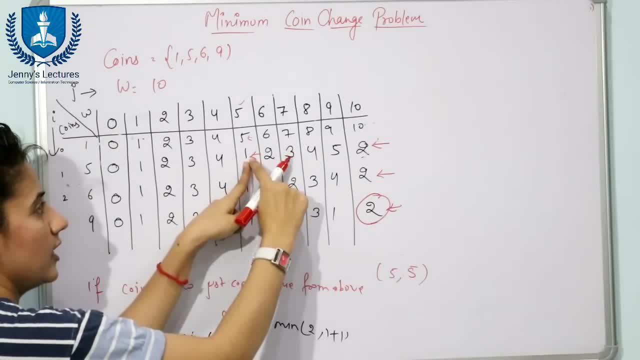 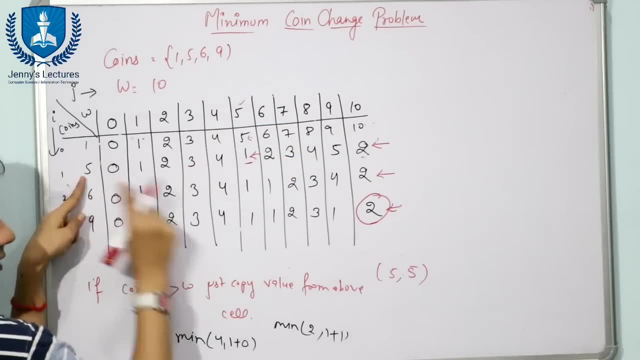 okay, now what you will do. pointer is here now. now check the amount in this column five. so reduce this five, because we have taken this five again. so just do five minus five and what we got zero. so in the same row we go to the column having value zero. so now we have reached to the column. 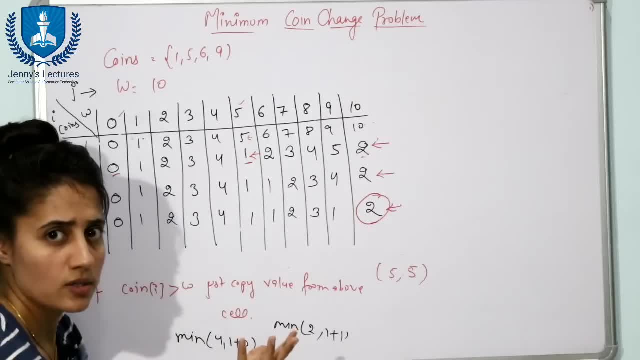 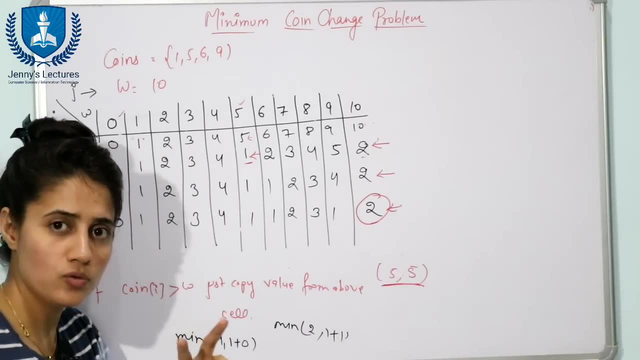 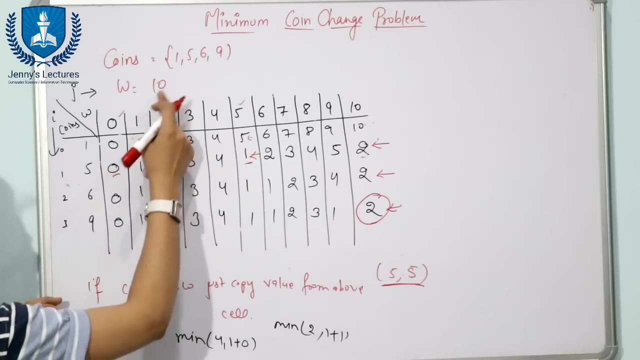 value having amount zero. so we have reached to the initial stage. now we are going to, we are not going to choose any point. so you can say five and five, two coins you will choose of same denomination and denomination is five and from this denomination also you can easily say to make a sum of ten. minimum number of coins needed is: if you we can take two coins of denomination five, then it will take some ten and that would be the minimum number of coins. okay, so this is how you are going to find out coins of which denomination you will take to make the sum. now, how to write the denomination of five. 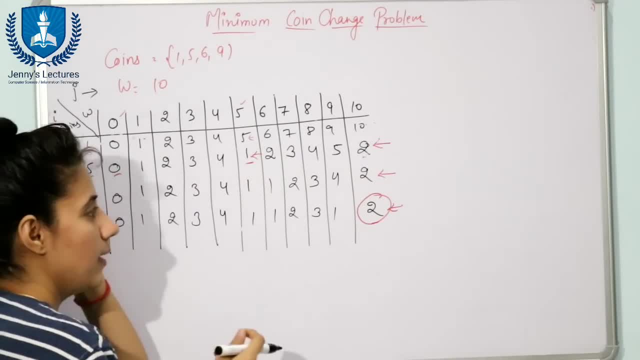 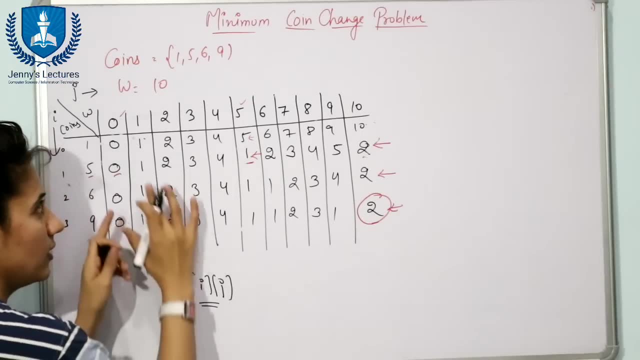 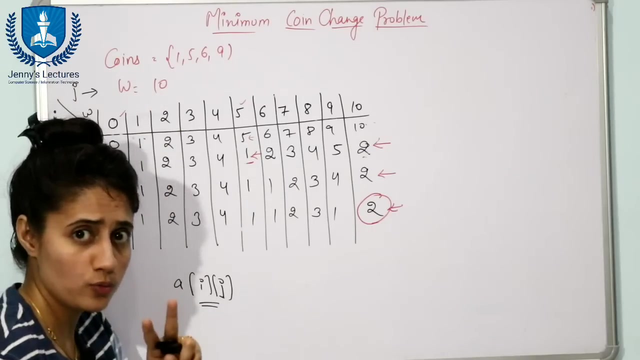 you can write down this logic. see the same array i am going to take. array name is a and i and j. a means we are a 2d array i am going to take, in which this these values are to be stored: i for this and j for columns and for two for loops would be applied first of all, what you will do. 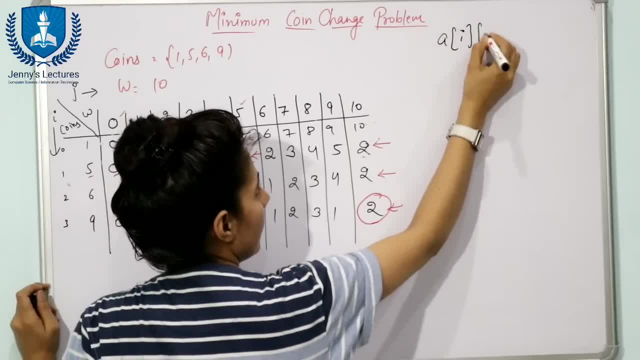 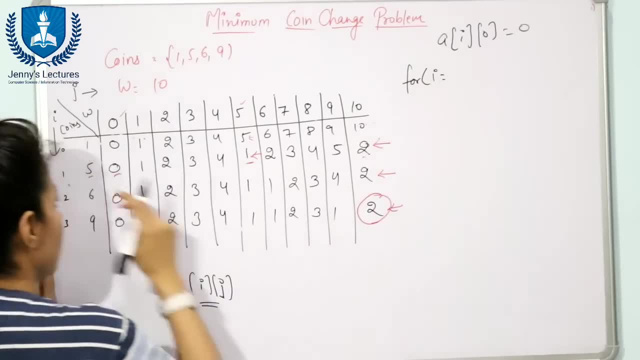 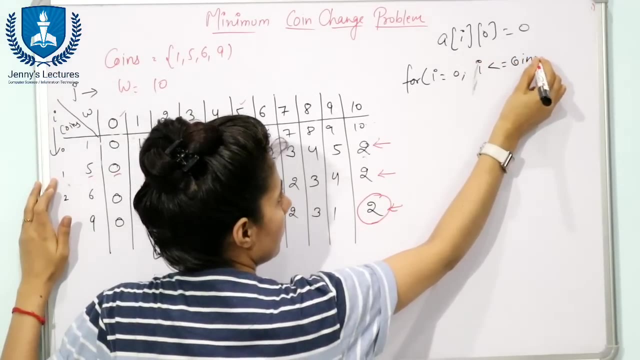 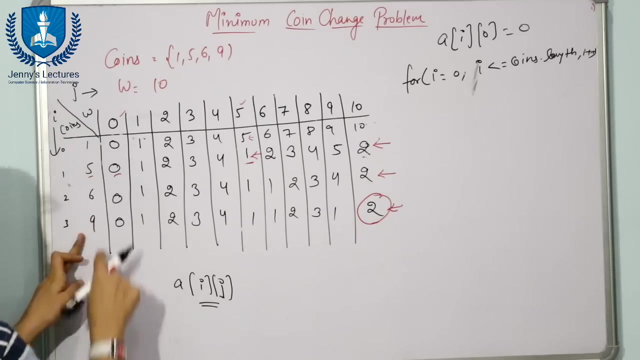 you just do a of i and in a zeroth column we just put zero. now for loops would be applied first of all for rows. j is equal to zero, to sorry, i is equal to zero. i is less than equal to coins dot length. you can say: and i plus, plus see. coin says the name of the array, so coins dot length. 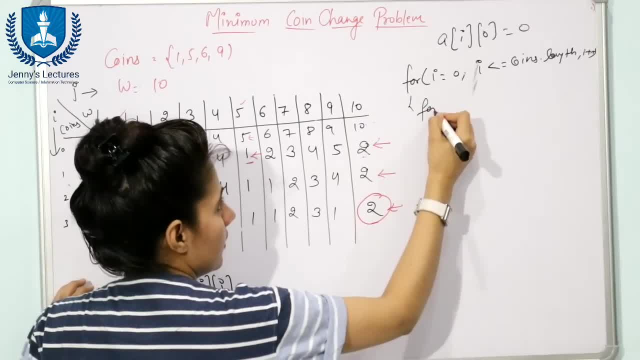 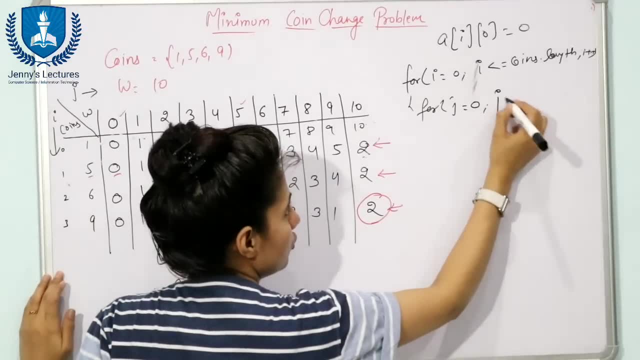 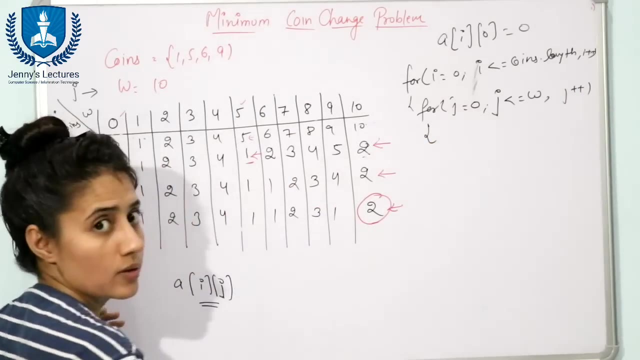 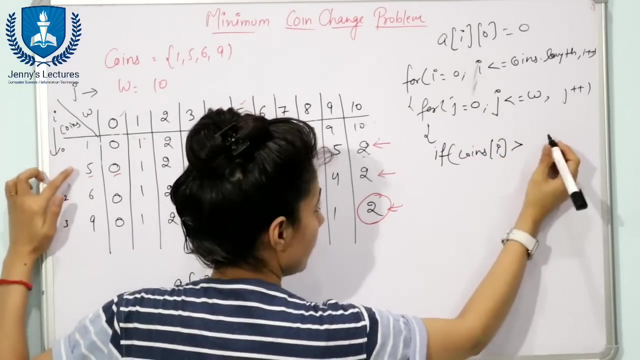 okay, now i plus plus. now, in this loop, one another for loop would be applied for this: columns j should be less than equal to this w and j plus plus. now here you will check what if the coins this, this value, is, this value is greater than this j value, then what we have done, simply copy the value from the above. 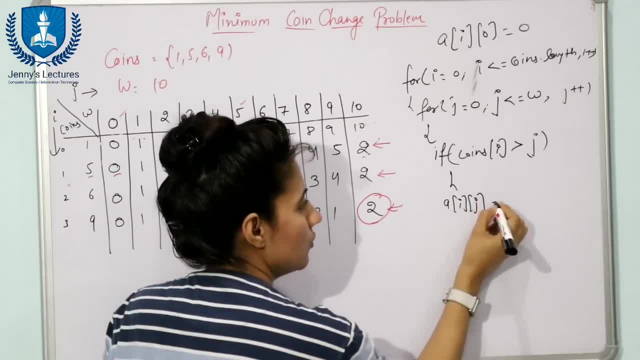 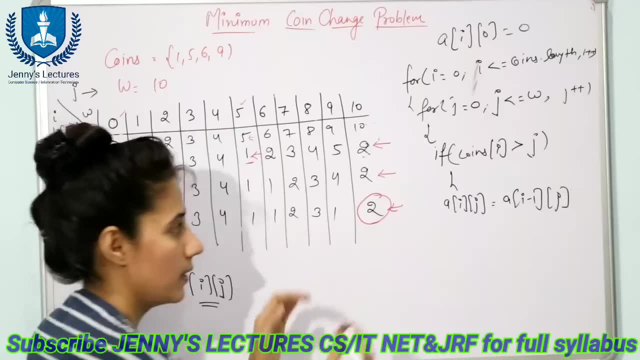 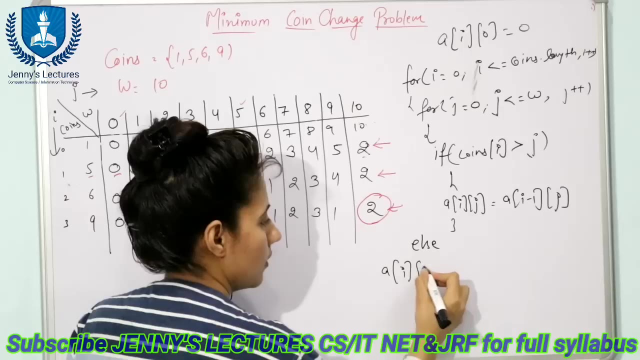 cell. so now a of i of j would be a of i minus one and j i minus one above cell but column would be the same. but if this condition is not true, then what we have done is we have taken a of i j to be minus with i plus three. i of one, a of i j would be. you have taken. a of one j, 2 i of one. a of 3 of a minus 3. 1 a of one i j n minus 3. one j, 2 a of a 2 i j y plus 1 j. reopened a of i. j mean a of j would be number two, number one a of i j would be. 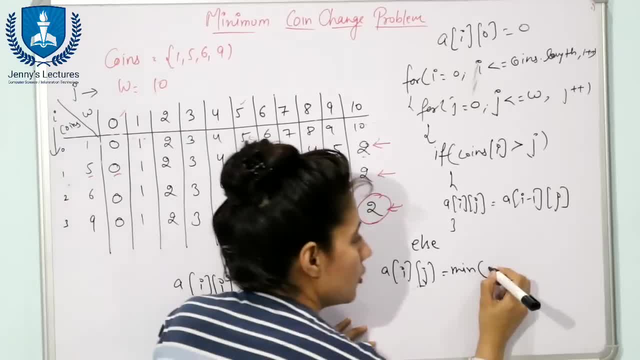 愛 inj would be c, to be minus i of j, un radical value minus one. but you can also balance it with a minimum of first one. all this interval time i of j, j would be minimum of the value from the above cell. so a of i minus one j and second value. we have calculated how: 1. 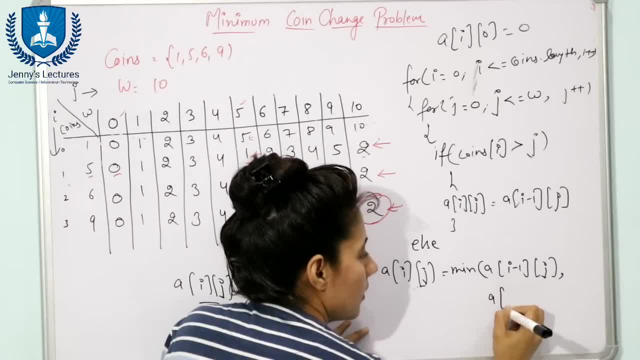 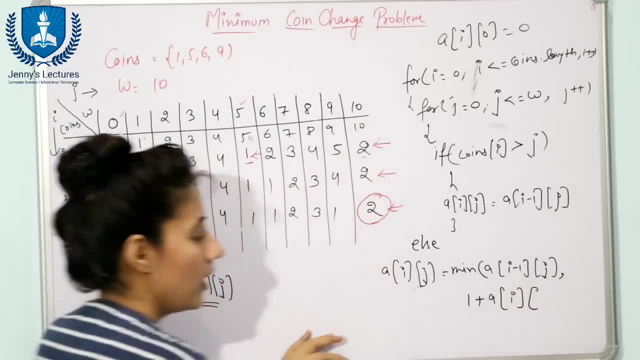 plus one plus a of i row would be same together. consider it: a of 1, a of j minus 1 by r greater, or multiply by half i to the power of zero by r, equal to zero. i minus i minus j. j would be as a of i row would be same, but we have just reduced this value from the column value in that.